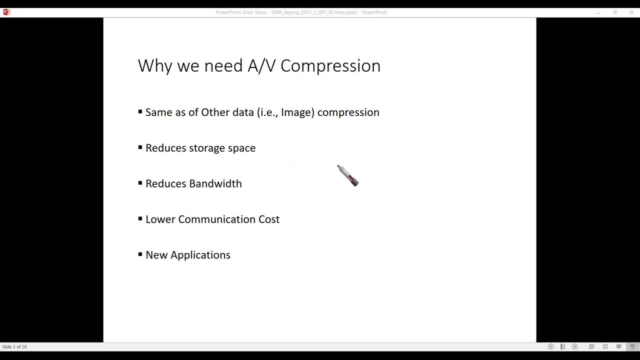 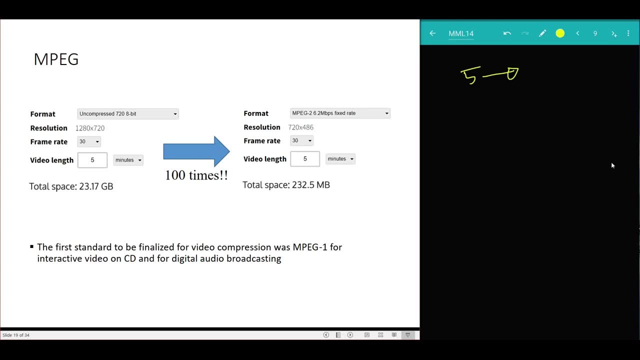 compressions. I explained this slide you know earlier when we started audio compression, so no need to repeat that again. Video compression: see that why and how this. this is useful and I'm sure that you you are already familiar this sort of idea, So see here. 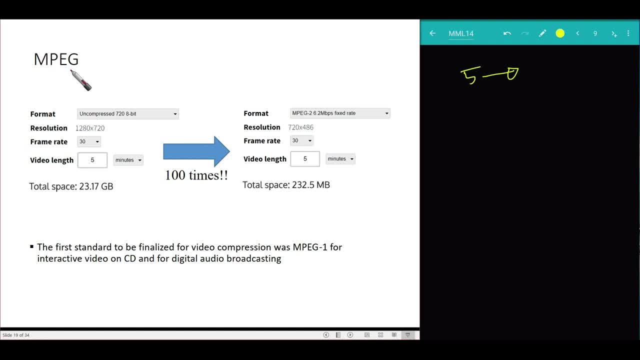 that you know MPEG right. Let's say we see the capacity of MPEG. MPEG, as I told you, is moving picture expert group. This is a standardization group and they worked very much, you know, on audio video and also sound. So this is a standardization group and they worked very much, you know, on audio. 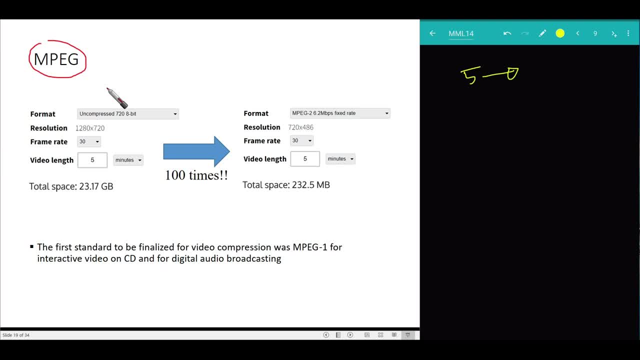 video and also sound. So this is a standardization group and they worked very much, you know, on audio system sound. So now we already talked onMPEG audio, now we'll be talking on System sound. So now we already talked on MPEG audio, now we'll be talking on. 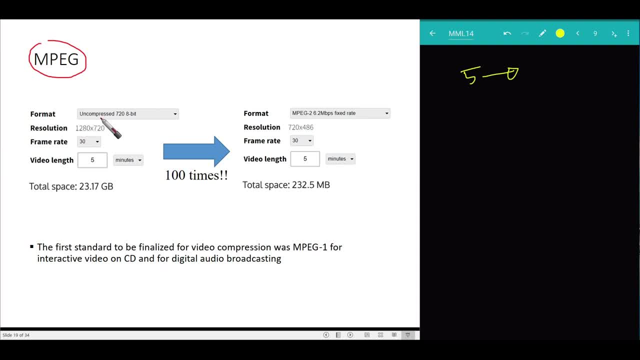 video. So see that if we have, let's say, uncompressed, you know data for examples, video. So see that if we have, let's say, uncompressed, you know data for examples, let's say, where the frame size is 1280 x 720 pixels. So that means you know kind. 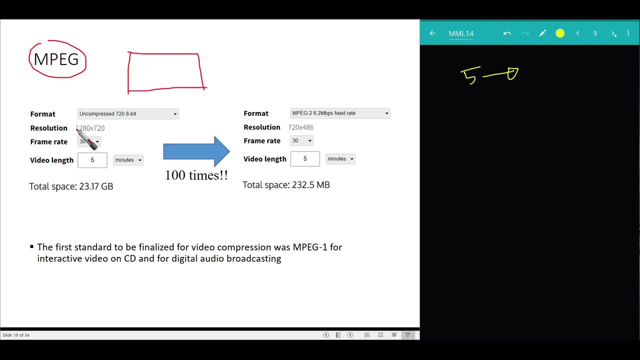 let's say, where the frame size is 1280 x 720 pixels. So that means you know, kind of, you know these kind of pixels right. Let's see horizontally, we have, you know, 288 pixels and our image height, or the frame height, more appropriatelyそうですね. 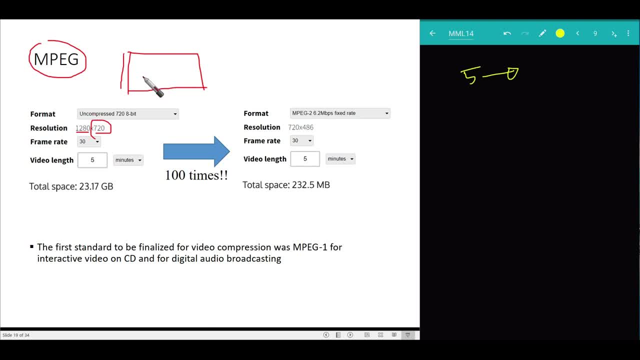 720 pixels. and and what is video? video, basically, you know the sequence of frames, right, it's nothing other than that sequence, it kind of sequence of image, and and then there are, you know, you know, let's say, 30 frames per second. and if 30 frames per second, and, and each frame size is this one, 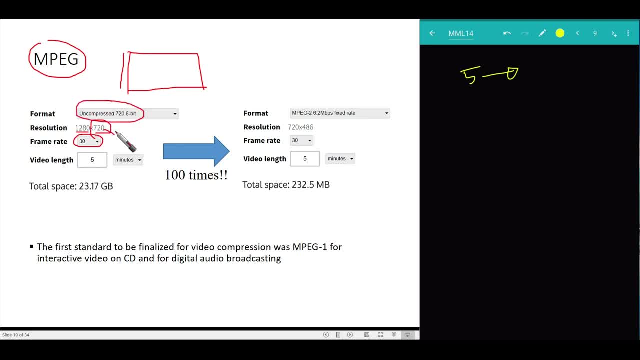 and if we have uncompressed, you know video, kind of this, and you know, for sansay video, for five-minute video we need almost 23 gigabyte stories. so see, for five-minute video we need to 23 gigabyte video can imagine. but if we just, you know, on this uncompressed video, if we apply, 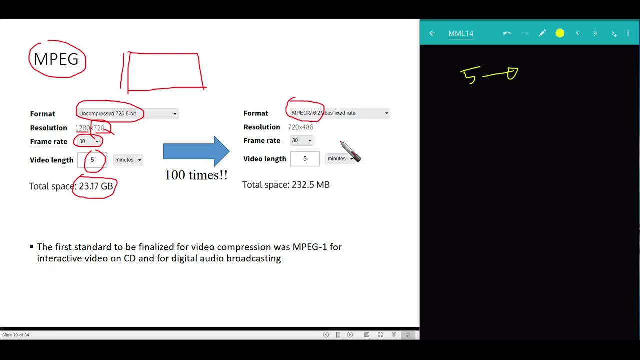 let's say mpeg, you know to, in a kind of, you know, from some sort of mpeg compression you and just a little bit, you know reduced, that's, the resolution is a little bit reduced. there's a 720, you know, by 486, and we keep the same frame rate and with this compression the space now become. 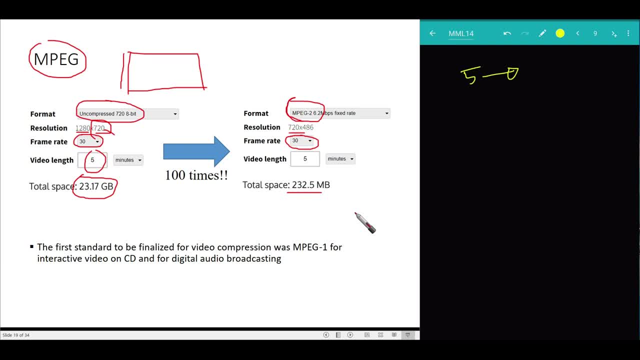 you know 232 megabyte only, so see 100 times. you know reduction compressions happening and this is happening and that's the you know that's the need and that's the importance of why we need video compression. so first standard, you know that was finalized for video compression was in peg one. 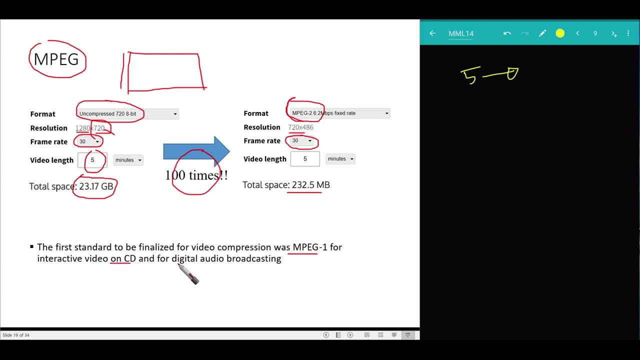 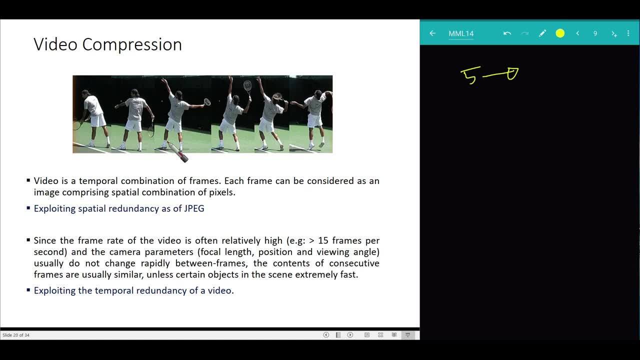 for interactive video on cd and for digital audio broad broadcasting. but we are talking about here, you know, video, so video compression, you know what is the basic idea. so, if you see, the video is basically the sequence of the video and the sequence of the video and the sequence of the video. 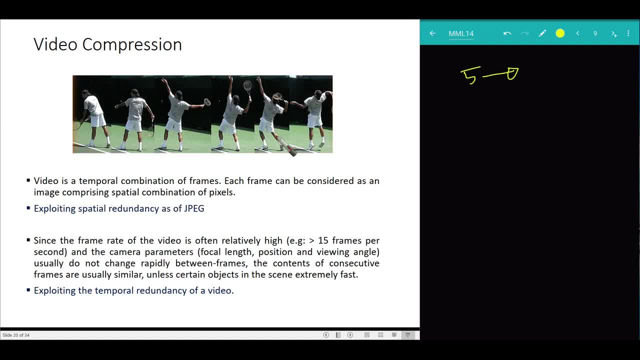 some image. see for examples here, these, these players that some action is doing and and, and you know these are some. you know consecutive frames, you know what we see, you know you know over over the time, but definitely from here to here is is is just, you know few milliseconds, not even. 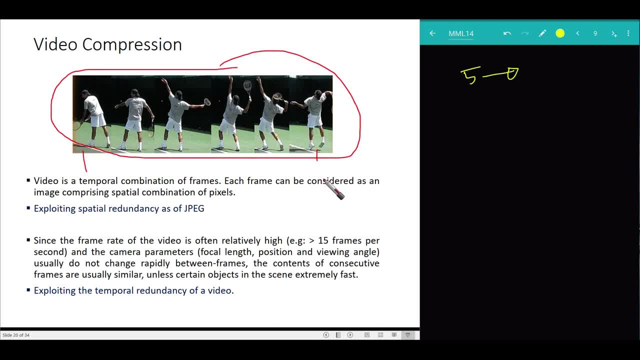 seconds, because at every second there are generally 30, 20, you know frames, frames, right. so that's why you know one second there are 30. you know such kind of you know frames, so definitely you know. you know, if we just see every frames, if we just, you know, keep every frame one by one, that we will see these. 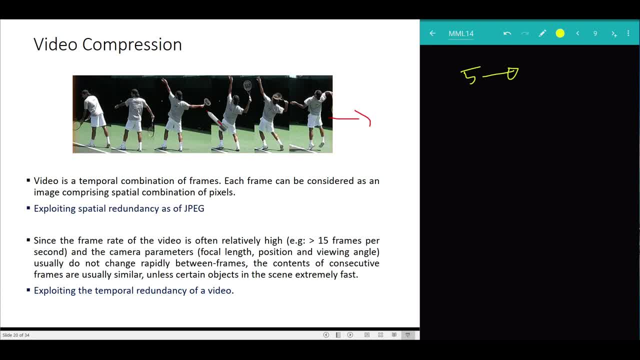 kind of things right where we can closely see and when this video replay- definitely quickly replayed, you know uh- before our eyes. so we can't, you know, differentiate between still image and the moving, you know, picture. so ultimately, what we are, you know, saying that's video is basically temporal combinations of frames. what is temporal? temporal means, you know, time. 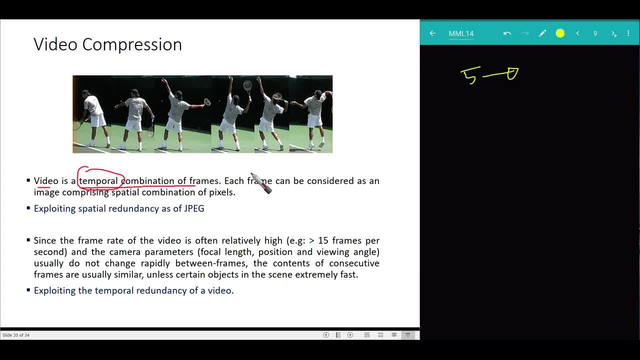 right temporal combinations of frames and each frame can be considered as an image, right? for example, like, like, like, like this one, let's say this image, this single image, or let's say this single image, so this single image is, ultimately is is kind of we can say this is a kind of jpeg image, right, kind of you know, one single image is. 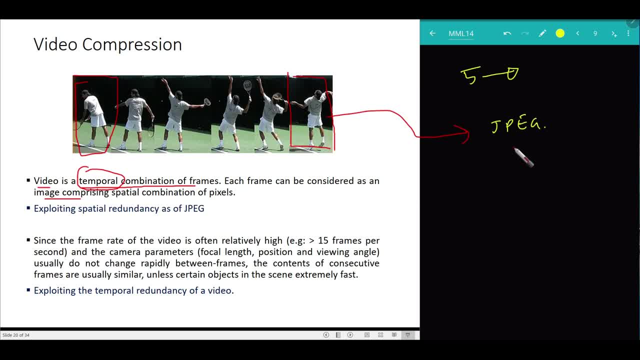 kind of jpeg image and definitely, you know if we have one, you know image, you know if we think about only one image, one jpeg image, one jpeg image itself can be compressed right as you, as you know, that from our image compression using jpeg compression, that one image itself we can. 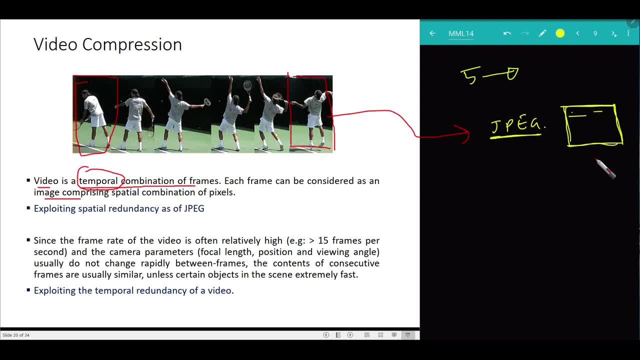 compress and and there you know, because that, how this you know the pixels are, you know distributed pixels are there and we use some dct compression techniques, then we used that one right. so for when we talk about just on a single image, that compression is still possible, but when you know, 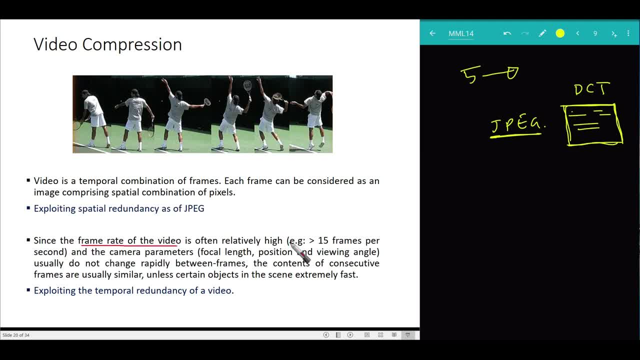 see that you know, we generally the frame rate of video is very large, right you know, usually greater than 15 frames per second, even 20, even 30 frames per second, even 60 frames per second, right? so where you know, just you know the camera meters. for example, now, when you take a video, we usually don't change focal length camera positions. 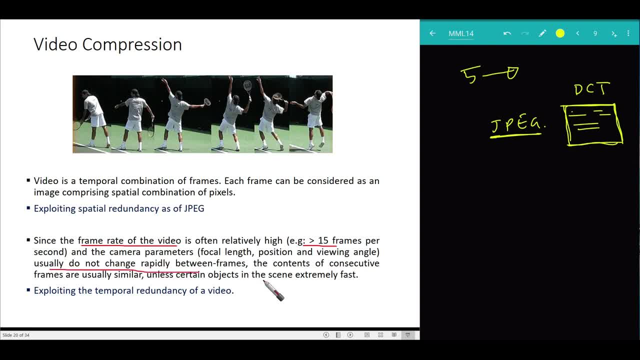 viewing angle. you know we do not change rapidly from frame to frames. right, so what? we can see that in consecutive frames, from this frame to this frame, the most of the, you know, things are almost equal. so some object might move, for example, here hand little move, maybe ball or this you 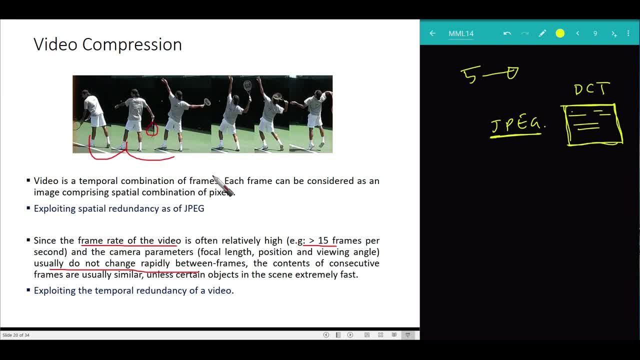 know bat might be moving towards. so what we can do is, basically, we can exploit the temporal redundancy. what does it mean? temporal redundancy? there's a redundancy. you know the word redundancy. redundancy means xs, xxs, right, xs, additional, additional, additional, additional information. so so that means this frame to this frame, this frame to this frame. you know there are some you. 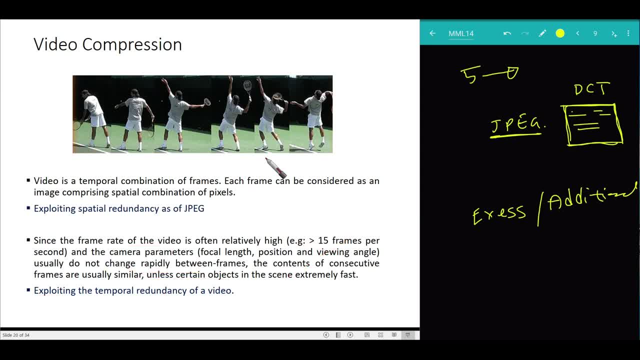 know large. you know part of this. for example, from this frame to this frame, a very large part between this frame to this frame. you know some xs, xxs, if we consider these frames, you know this, xxs are the same and those frames are same. so all we can say, you know, the same information are repeated, so 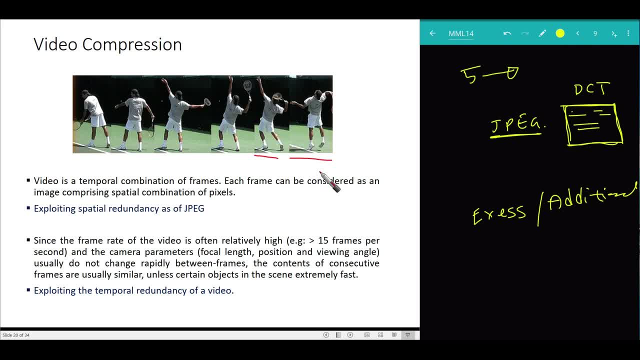 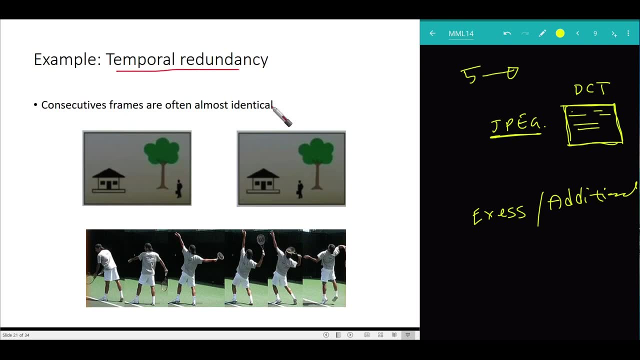 this is kind of excess information, additional information we don't need. we can just keep the same information once and the new information we can just, you know, consider so, so that is called redundancy, some additional information. and then when we look, you know, irrespective of time, temporal redundancies like that, for example, let's say these two are, you know, two consecutive frames. 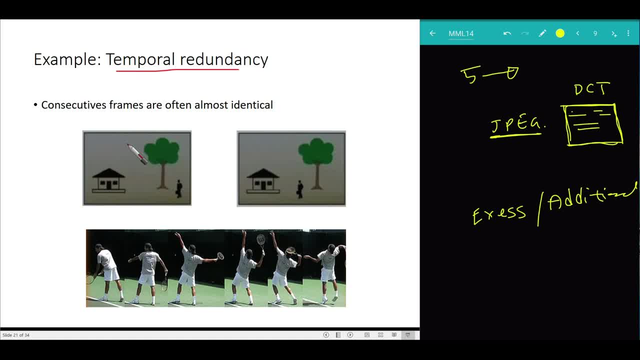 so in these two consecutive frames, you see, most of the things are equal, most of the contents are equal. these are equal, these are equal, this same information right. only things happen. this person, he was perhaps walking from here and he just little from from earlier. he was here like and. 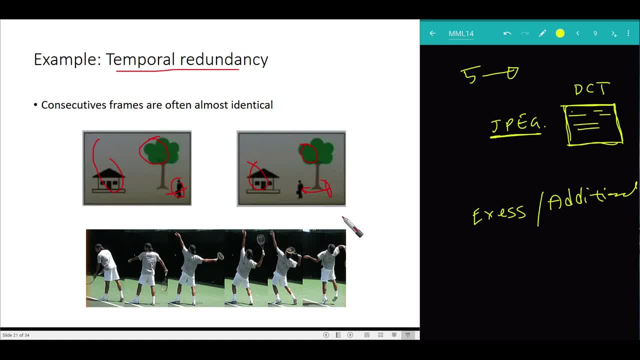 now, it's little bit, you know, forward and he comes here, right. so this is only the differences. now, how about? i mean, let's say that we- just, you know, transmit this information or we keep, only you know. we keep this information, but we don't, you know, send this information, this image. we only transmit. 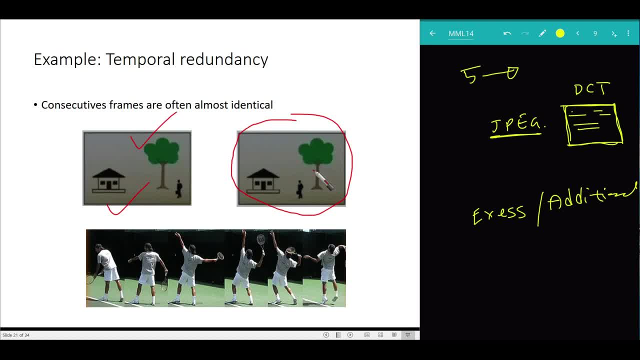 this frame, but we don't transmit this frame. rather, what we do, we just send the difference information only. this new information, we can, you know, keep or we can preserve, we can transmit. so add that, if we do this way, so that means we don't need to, you know, store this whole. 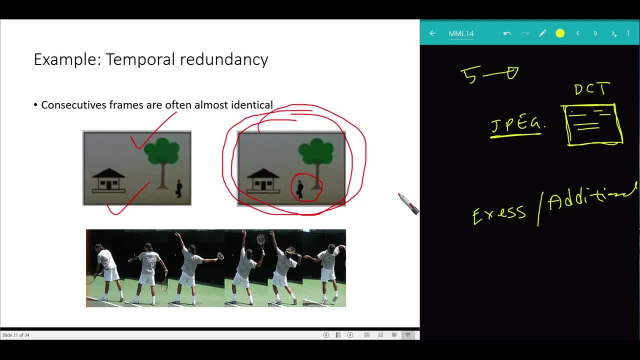 you know image right. so frame by frame we can compare and then we can keep some frame and with reference with that frame, the other frame we can regenerate, it, we can remake. so that's the idea of you know temporal redundancy, so we can exploit, we can use the temporal redundancy. 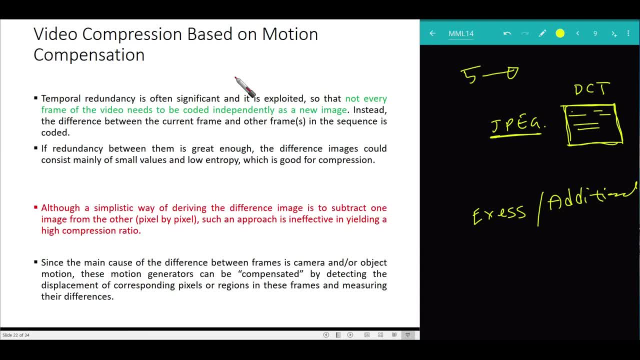 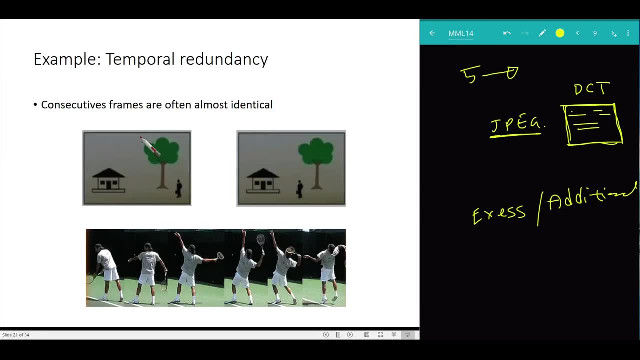 you know, to have, you know, our video compressed so- and interestingly, you know, temporal redundancy is often very significant. yeah, so, for examples, not every frame of the video needs to be coded independently. for examples, here let's say, you know, let's say, this is a jpeg image, we can just, you know, code and we can preserve. 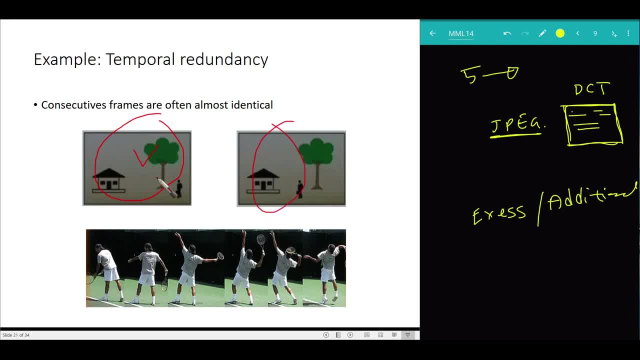 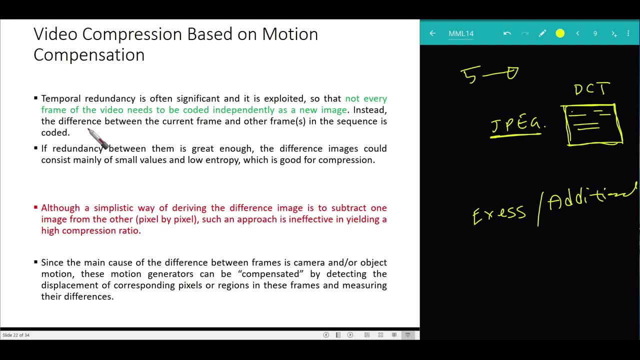 but we don't need to code this one right, because we already have this one and most of the information in this frame are similar. okay, so we just do some difference between the current frame and the other frame in the sequence, okay, so redundancy between there is really great enough. so what we do for examples you know, think about from information, theoretic. 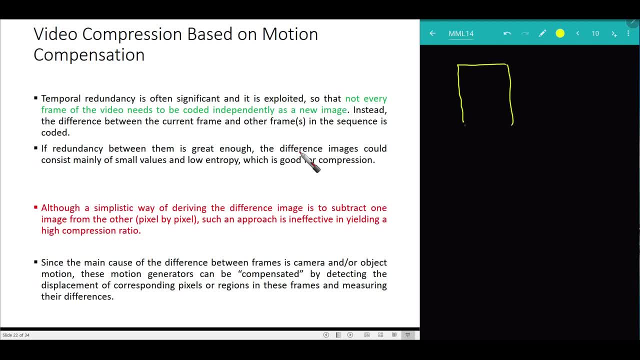 perspective. let's say one one frame is this. let's say this is frame number one and let's say this is frame number two. right, so we just transmit this information as it is, for example, like a jpeg image, or simply we just, you know, compress like jpeg image and so it is as it is. we keep as it is. 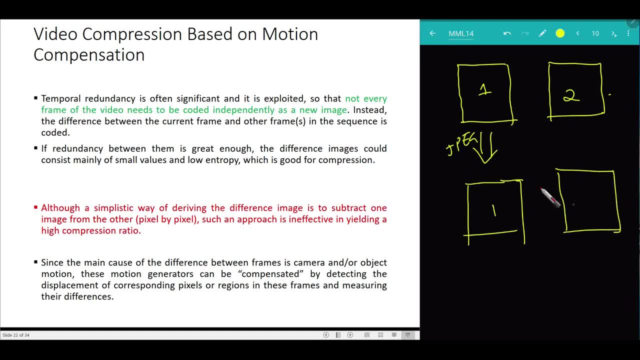 now, how about the next frame, next frame? what we do is, let's say, we just do two minus one. so when we, you know, we send a frame, but this frame basically a difference image, we can say: this is a difference, difference image. why i'm saying difference image? because we are just, you know, having pixel by pixel. 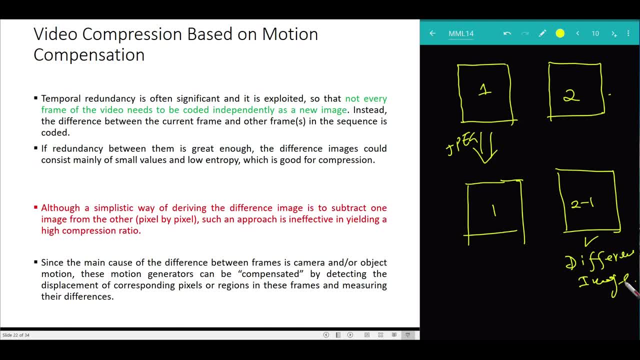 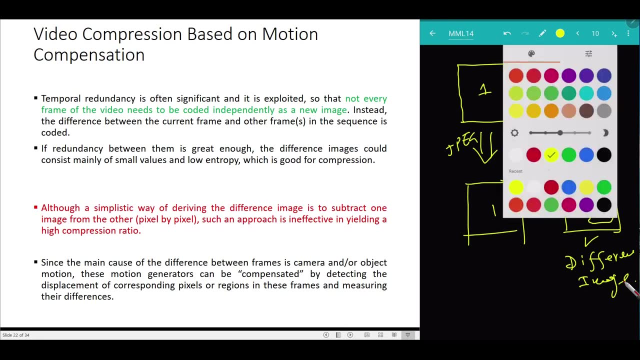 differences. let's for this time b. okay, so this is the difference: image two minus one. now, when you do the differences, so what will happen? most of the pixel will be zeros or at exactly very low values: zero, one, something, something, something and just few pixels, maybe in this region, maybe in this region, in this region, maybe some values will be like you know. 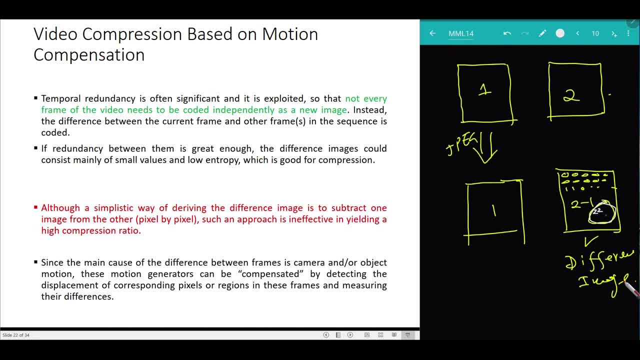 a lot of changes, maybe maybe 23, maybe 100, something, something right and or most of the, because this is a difference image. so this is basically two minus one. two minus one, so most of the values will be zero. and because most of the values will be zero if we do some, you know, run. 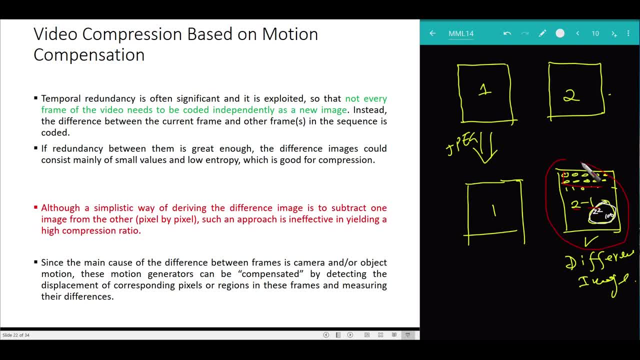 length, coding or something, then we, this image will be reduced a lot compared to this one, right? so this image will be reduced a lot. so that's the idea that how we can apply, you know, the, we can utilize the redundancy, and then you know we can compress the video, but definitely, as it looks very simple, that we just you know. 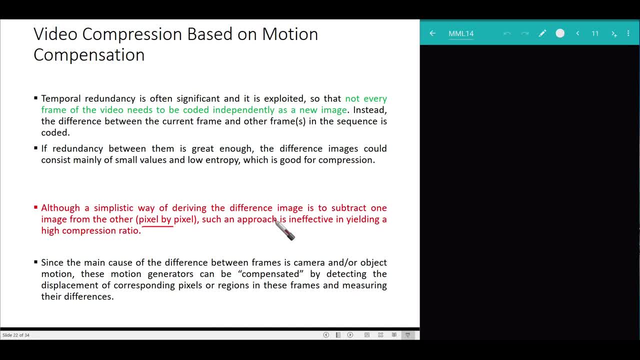 have pixel by pixel differences, but this is not very effective. you know this is basically ineffective for high compression ratio. we do some sort of other mechanisms. so, and as i told you, the main causes of the differences between the frames, basically camera and object motion. okay, now, definitely this motion, you know from image. 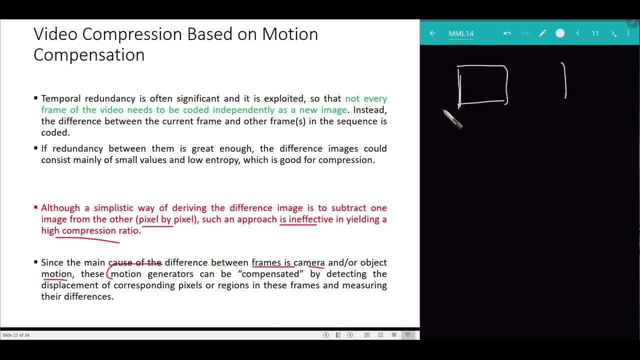 from when we go from this image, when you go from this image to this image, let's say, you know, there was there, there was. this image is something like: okay, but in this image some, suddenly an object might appear, right, so this kind of object, so you know. 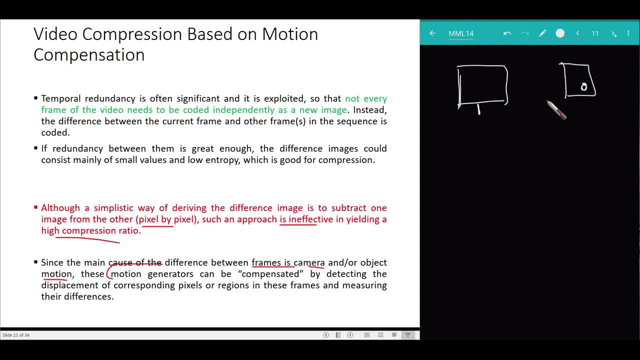 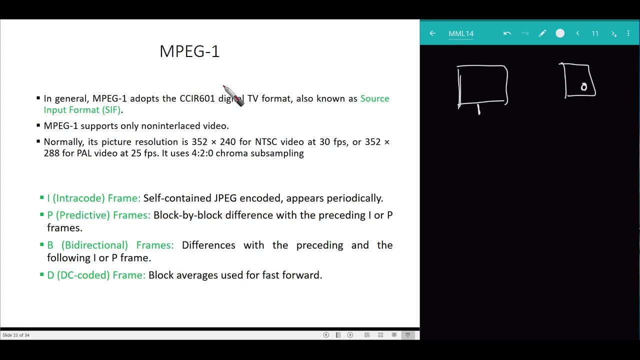 so this motion, that that in which direction some object is moving, so that kind of motion compensation we need to do and accordingly we say video compression based on motion compensation, okay, in mpeg-1, you know. so, uh, if we, if we think about the video we we saw the audio, if we think about 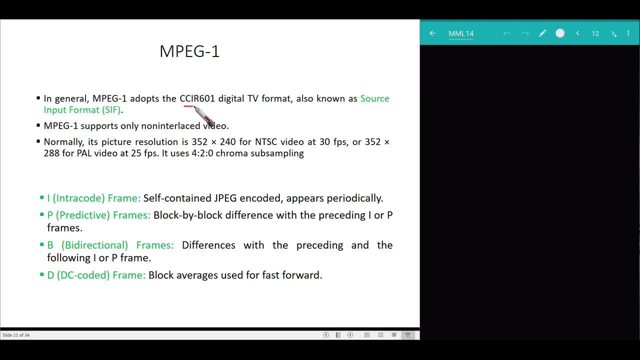 the video is basically adopts. you know kinds of, you know this kind of, you know digital tv format and sometimes we say this is kind of you know source input format. you don't need to know that. what is this? digital format is some sort of format, so mpeg-1, basically you know it. 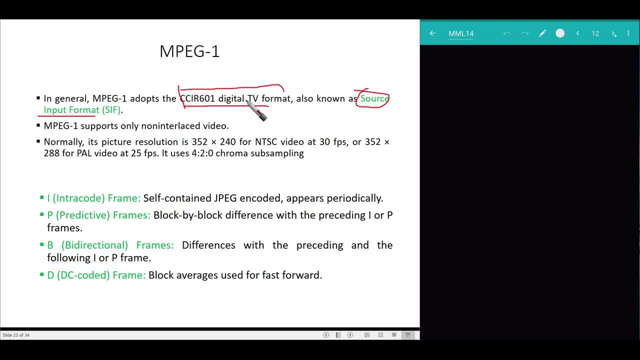 borrows some concept from this. you know, uh, you know television signal formatting and the best known for you know, source input. for me this is kind of format, or we say s i f for me, zip for me. and mpeg-1 supports only non-intell list video. it doesn't. 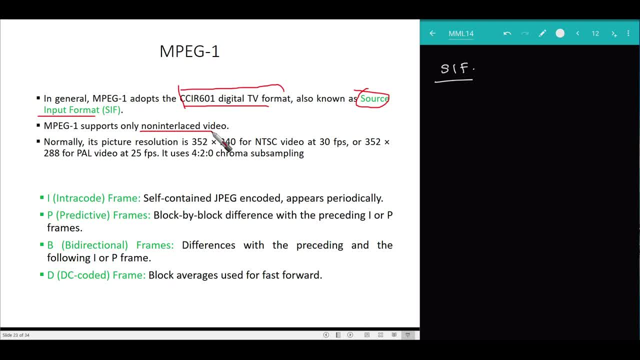 doesn't, you know, support interlaced video, if you remember that what is interlaced or what is non-interlaced? and the picture resolution is actually, you know, very low. in fact you see 352 by 240. you know image size for NTSC video. now, why are you talking about the NTSC, if you remember. 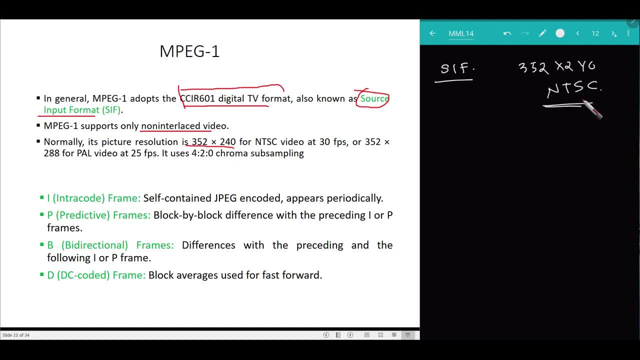 that I talked about NTSC, because it's, you know, national television, eastern committee, because initially the MPEG-1 was targeted for digital TV and it used, you know, 30 frames per second. it also used 352 by 288 for PAL video and you know the PAL is also television signal phase. 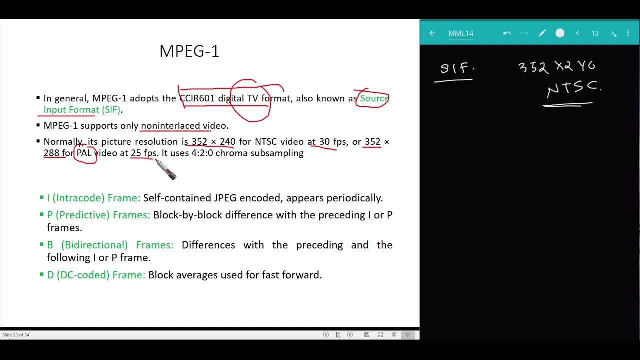 alternative, alternative line video and in 25 frames per second and it uses this kind of chroma subsample. so this is very much. you know some. you know kind of description of features, so how MPEG-1 works in MPEG-1. you know, if you remember that you know the video means a sequence. 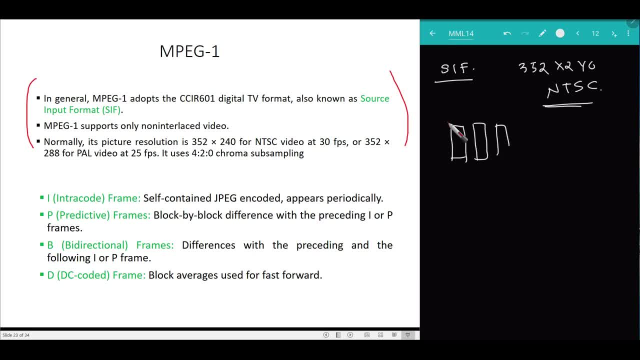 of frames, right frame one, frame two, frame three and in this way, okay, so MPEG. so what? what it does is is basically, you know, designate and make some specific, you know kind of frames. for example, in MPEG, some frames are called MPEG-1 and some frames are called MPEG-2 and some frames are called 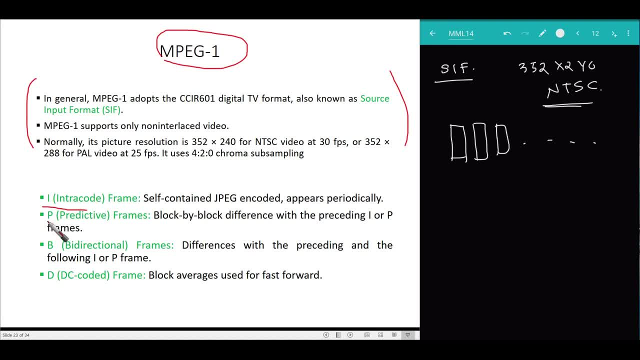 I-frame and some frames are called P-frame and some frames are called B-frame and some frames are called D-frames. so there are four different kinds of frame. so I-frame it's coming from intra code frame, and D coming from predictive, B coming from bi-directional and D coming 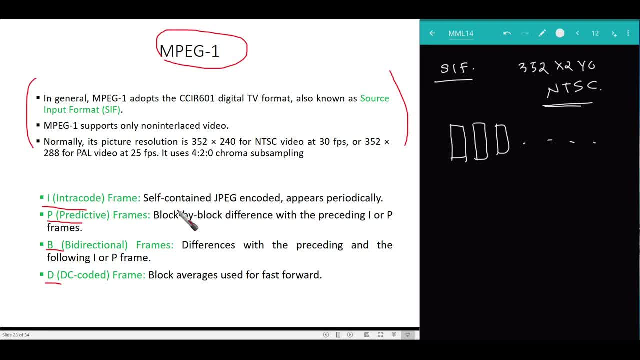 from DC coded frame. okay, so what is I-frame? I-frame is kind of, you know, self-contained, you know JPEG encoded image, for example. this is, I mean this image, this frame, let's say, if this is an I-frame, this I-frame is, you know, is standalone frame, it, this frame doesn't depend on any other. 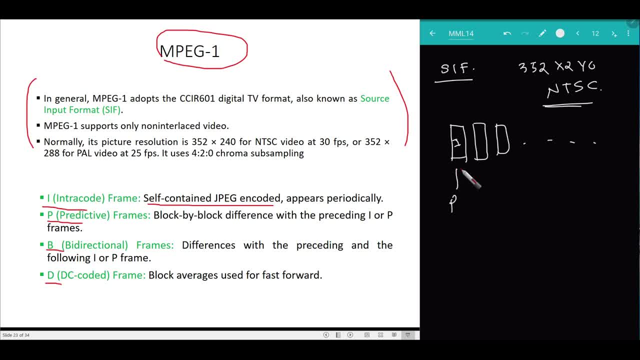 frame. this is also, we can say, this is the reference frame. okay, so that means you know, periodically, you know MPEG, what it does is periodically it sends an I-frame and then some other frame and then again I-frame. okay, so this I-frame, you know, doesn't depend on any other frame, so that means it can be decoded. 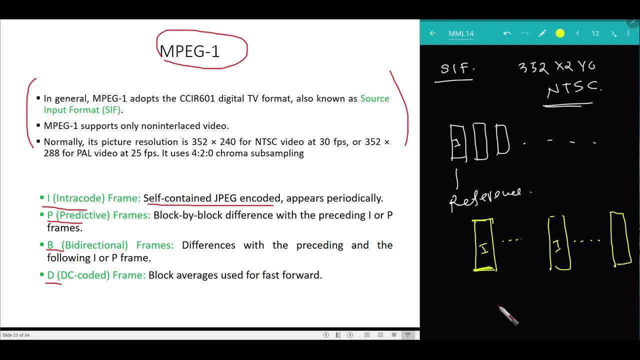 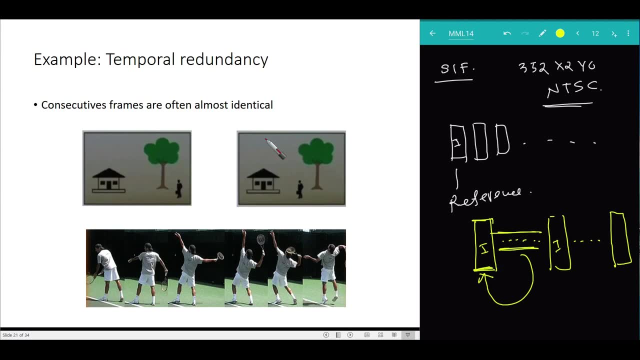 encoded just independently, okay, and but other frame you know will constitute, will recover other frame with reference to this I-frame. so that's why I-frame, basically reference frame, so you can think about like this: you know, let's, if you go back here, for example, if you think about this: 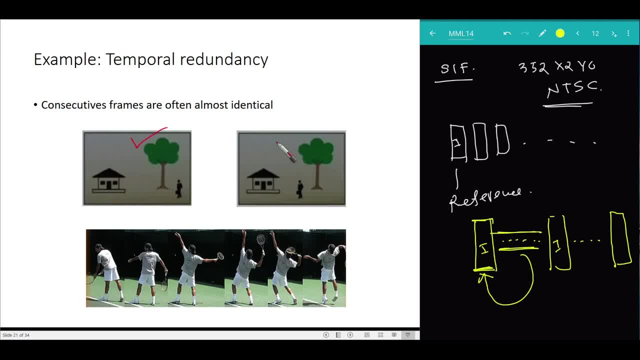 is I-frame or reference frame, then? and then this is a difference frame. maybe this is not I-frame, so, but this frame can be generated, you know, with reference to this frame. so that's why we need to periodically, you know, send and periodically insert some sort of reference frame. so because you know, periodically, let's say, 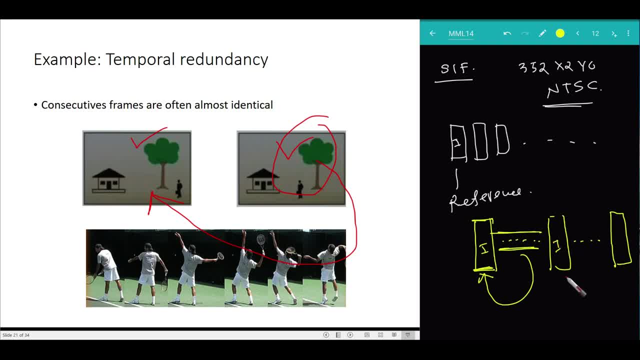 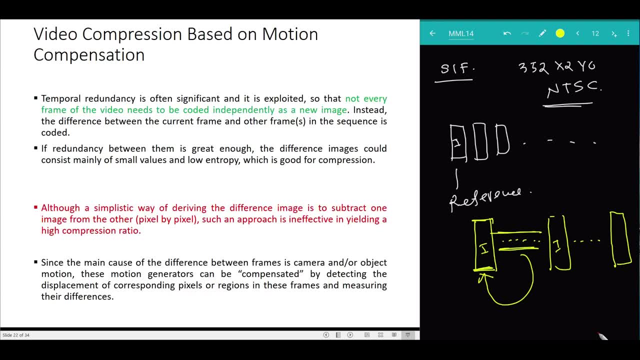 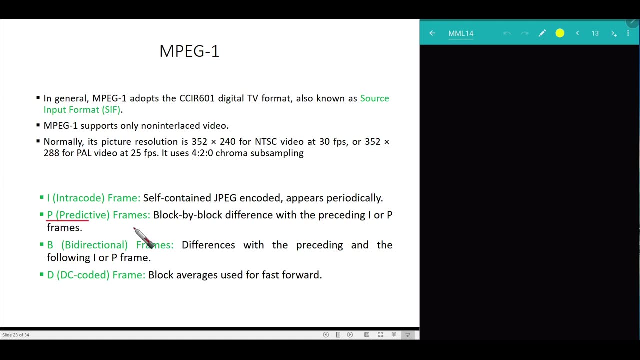 some other frame and then I-frame, so the other frame can be, you know, can be constructed from I-frame. so that's the idea. what is I-frame? So not only I-frame, the MPEG also have, you know, P-frame, that's called, you know, predictive frames. so that is block by block, differences with preceding p or I-frame. 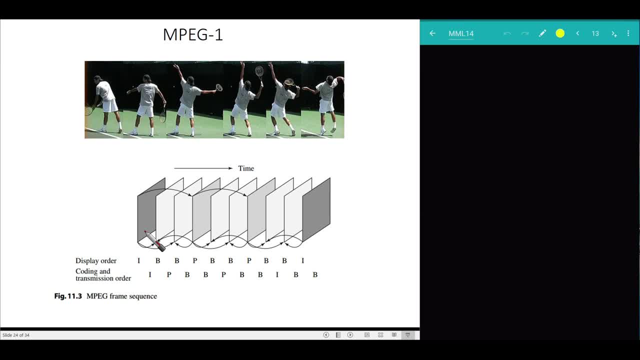 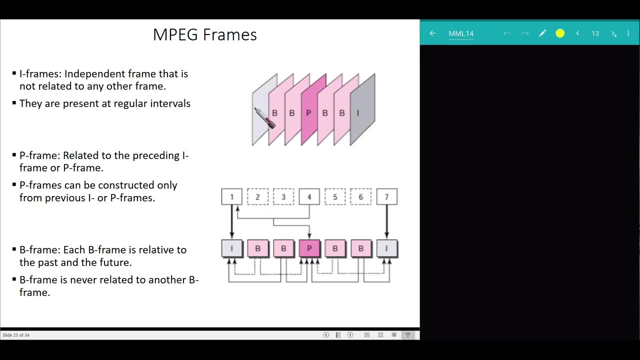 Okay, let's think about more appropriately like that. okay, so for examples like this, okay then let's say, let's, how about? this one is kind of this, kind of things. let's say: this is an I-frame, and then you have one B-frame, 2 B-frame, and then 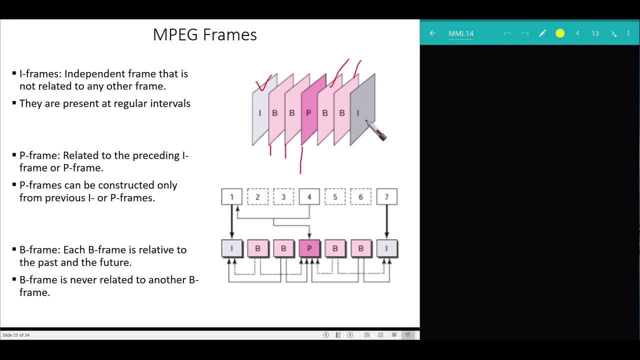 again you have P-frame and then B-frame, B-frame and then again I-frame, like this. okay, So this is kind of that how it works. okay, So independent frames, that is not related to any other frame And they are present at regular intervals, this I-frame, you see. 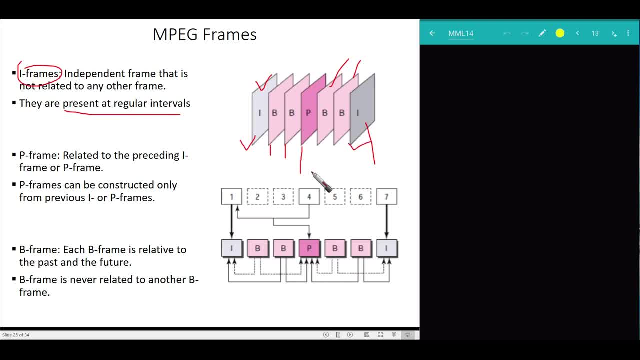 One I-frame and then other I-frames, something like that, And the P-frame is interesting because it's related to preceding I-frame or P-frame. That means, you see, this is an I-frame. Forget about this one right now, but think about this P-frame. 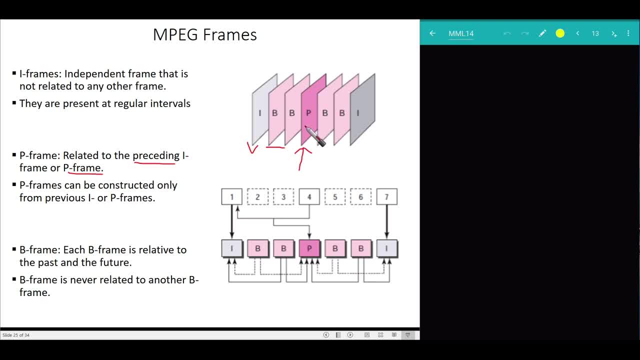 This P-frame can be, you know, generated, can be constructed, can be recovered, you know, from I-frame or P-frame. So generally I can draw here like this one kind of things. Let's say this one is one I-frame. 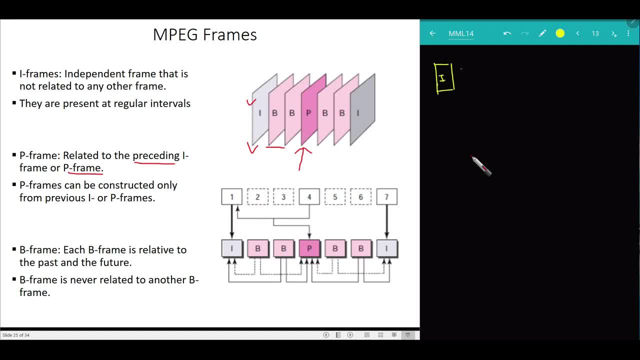 I-frame. And let's say, Let's say this one is, you know, maybe white color, This one is B-frame. And let's say I have now P-frame. And let's say again: we have B-frame, Okay. And let's say, now we have again one P-frame. 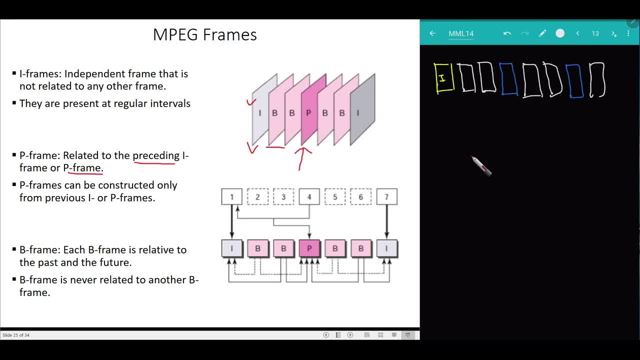 And then let's say again, we have some B-frame, And then again we have, you know, let's say, I-frame. okay, This is I-frame. So you see, this one is we can say, this one is P-frame. 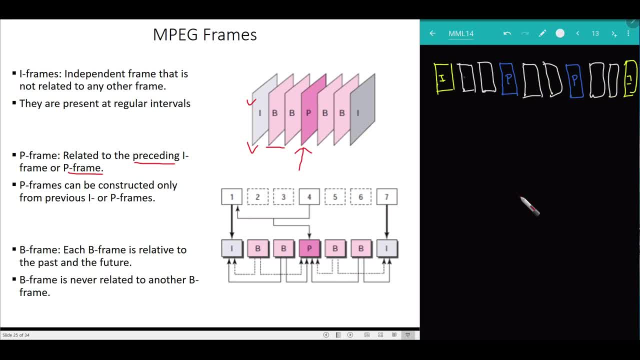 This is P-frame And all other are actually B-frame. Let's say, this is B-frame, B-frame, B-frame, B-frame, B-frame, B-frame. So this I-frame is original image. okay, This original frame. 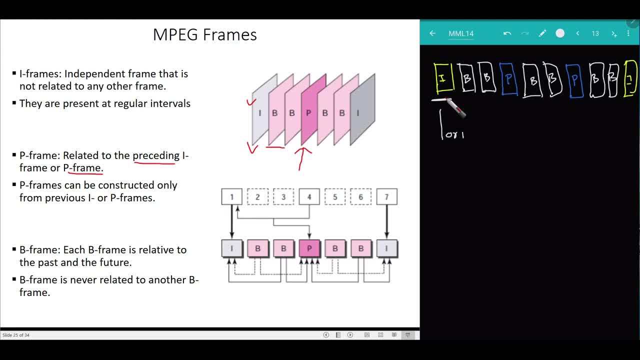 There is no compromise with this one. This I-frame is the original image, Original JPEG frame. You can say JPEG frame, JPEG frame, And then you know this P-frame is also constructed with some references, With references. this I-frame, you see. 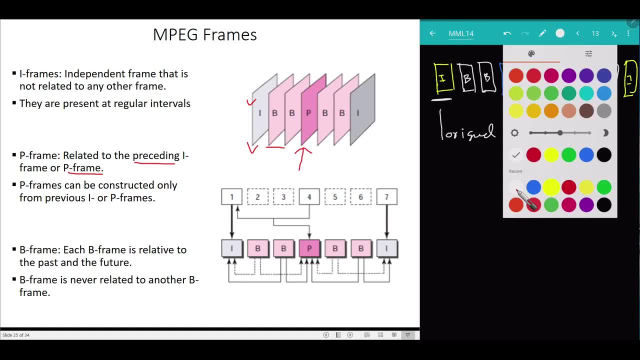 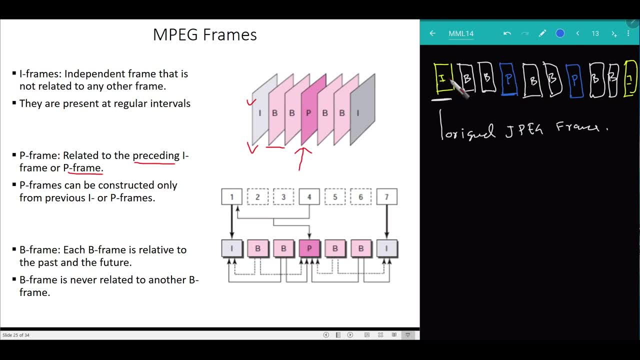 So that means you know, we don't, you know sense. you know something like you know how to recover this frame. Let's say you know. let's say we transmit I-frame. This is a complete reference frame. 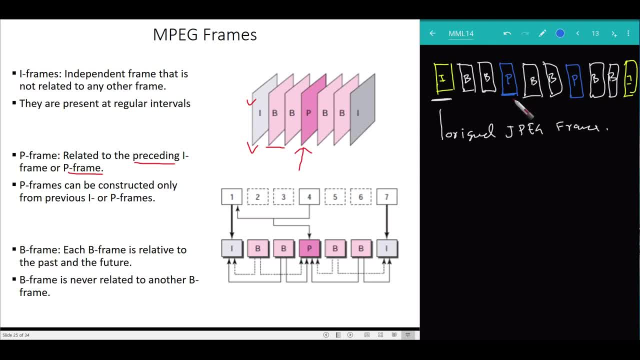 This is also a complete reference frame. We can say, this P is a semi-reference frame. So this P-frame, we can construct this P-frame from this I-frame. Okay, And how about this? you know this, you know this P-frame. 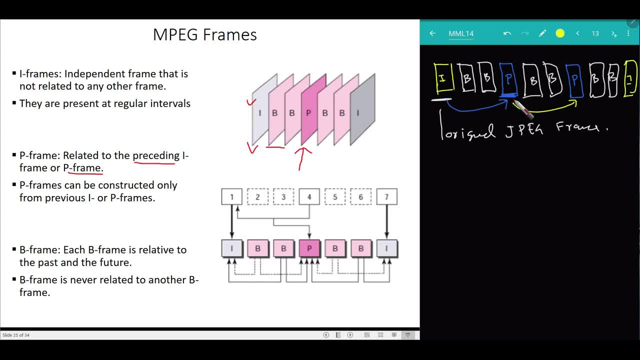 This P-frame can be constructed from this P-frame. Okay, This P-frame can be constructed from this P-frame. So it is also, it is, perhaps it is also you know these P-frames, maybe it is also possible to construct from this I-frame and this P-frame. 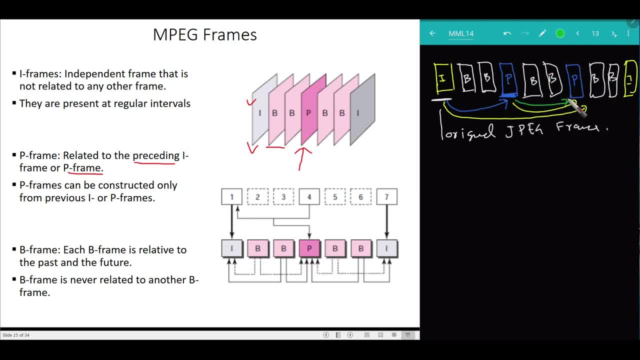 Okay, This is also possible from this P-frame. But what? whatever This P-frame, This P-frame we will construct from previous P-frame or I-frame? Okay, So, that is, that is the simple thing. And how about this I-frame? 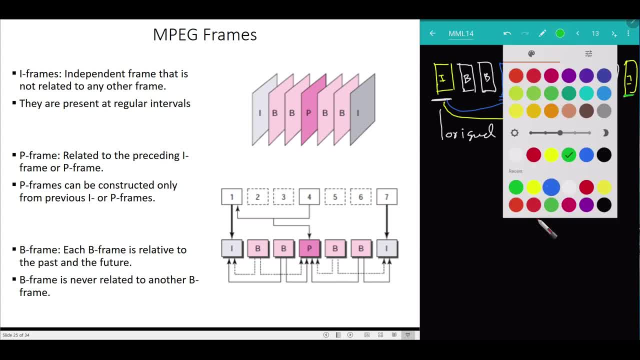 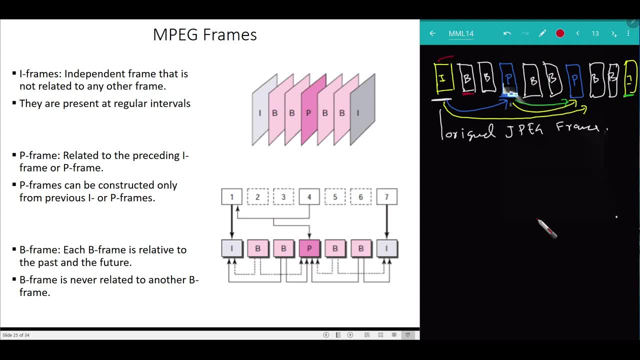 This I-frame is again independent. But how about this? you know, you know, I don't know, maybe there is red color. How about this B-frame? This B-frame will construct from this I-frame. This B-frame construct from this I-frame. 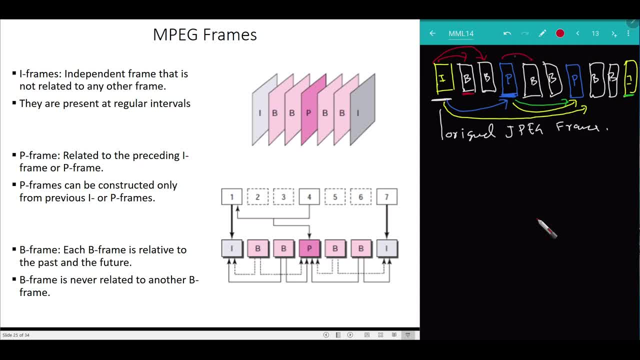 How about this B-frame? This B-frame is constructed from this P-frame- Okay, In fact it is. This B-frame is, let's say- I just make it simple- Like like this one. This B-frame is called bidirectional frame. 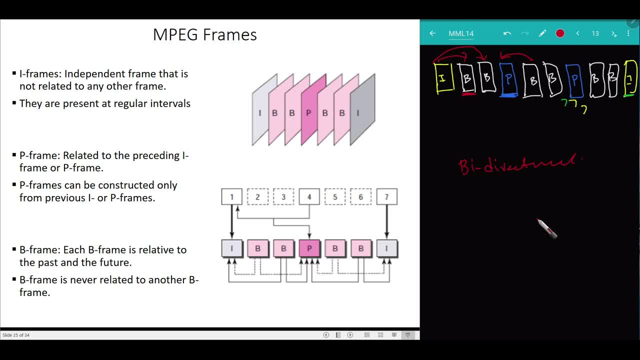 Why it is bidirectional. Bidirectional Because this B-frame not only depends on this I-frame, it also depends on this P-frame. Similarly, this B-frame is also depends on this P-frame and also depends on this I-frame. So, to construct this B-frame, we need both P-frame and I-frame. 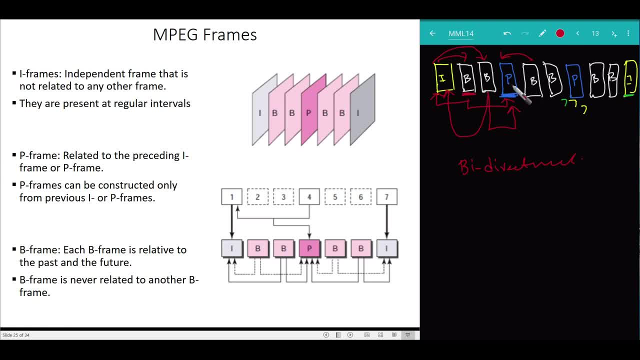 So, similarly, to construct This B-frame, we need this P-frame or this P-frame. So you see this B-frame sandwiched between these two P-frames. So that's why you know this B-frame depends on this one and this one. 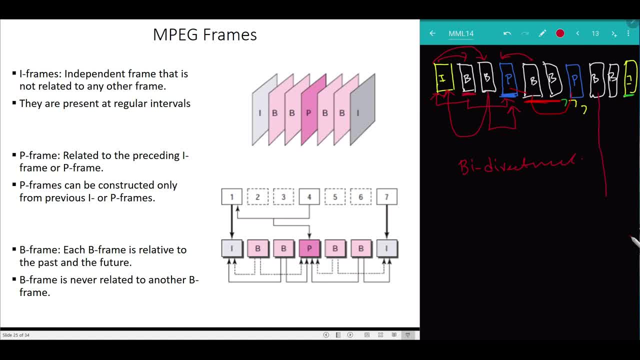 And how about this? you know, how about this B-frame? This B-frame depends on this P-frame and this I-frame. So this is how you know. you know the missing frames. we can, you know, regenerate, So so for. 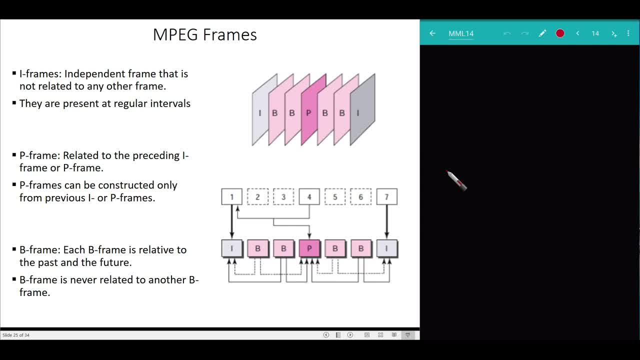 To make the, you know, consistency, to keep the track of our video. we regularly transmit some, We regularly transmit some I-frame And then, you know, with reference to this I-frame, we also construct some P-frame. And then, you know, with reference to both I and this P-frame, both I and this P-frame, we, you know, do some, you know, bidirectional frames. 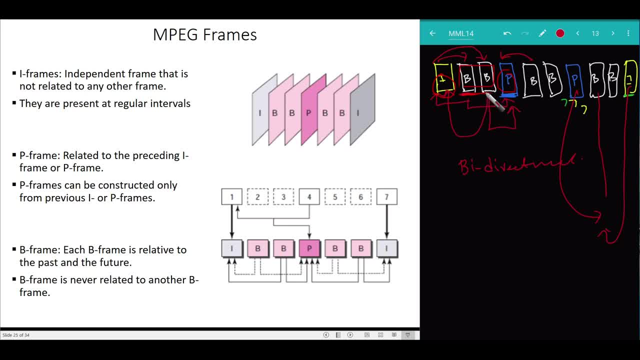 So these bidirectional frames to construct this bidirectional, these are. These are missing frames, right? We only send this I-frame and this I-frame as an independent frames. This is independent frames And this P-frames we send in reference to this I-frames. 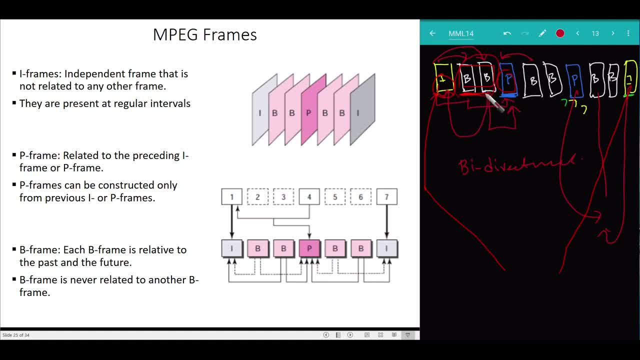 Now also, we send- you know this, you know- B-frames. This is kind of differences that constitute both this P-frame and this I-frame. So this is how we make it, For example, here look: 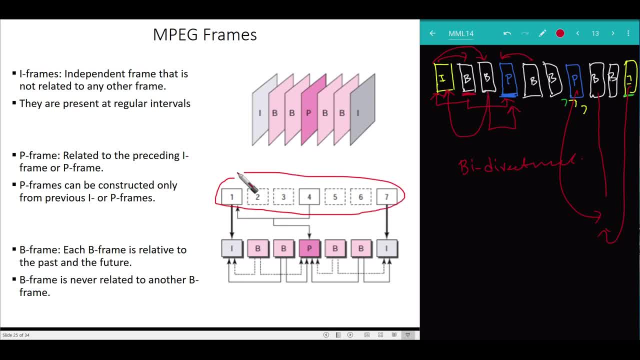 For example, let's say, this is our original you know frame. So we transmit this I as a very mass, this one. We also, you know, transmit this one, this I-frame And this P-frame. we also transmit this P-frame, you know. but you know we keep some you know references, you know, in reference with you know, maybe this P-frame depends on this I-frame. 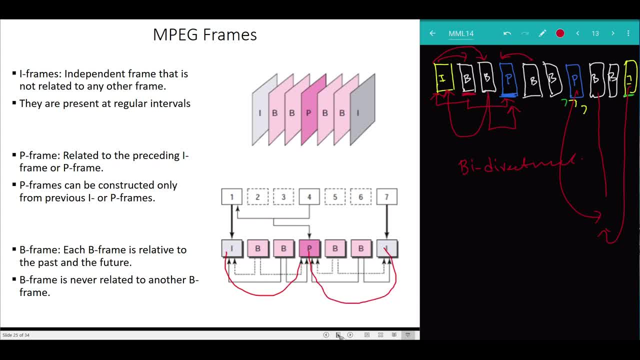 And maybe with this, you know, this I-frame And other frame, we basically don't transmit, Rather we regenerate this P-frame. with respect to This, you know B-frame and B-frame, So B-frame. how can we make this B-frame? 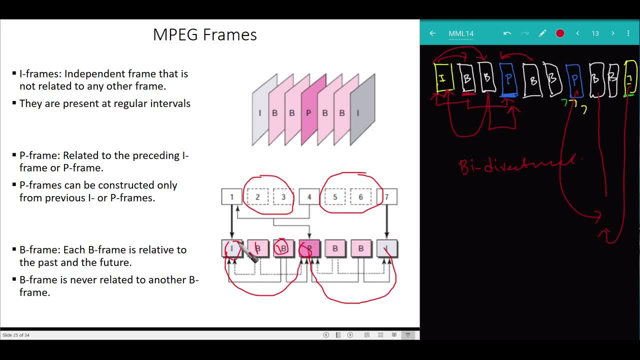 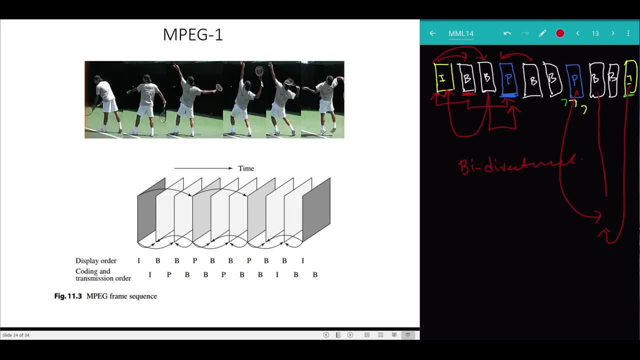 Using this I-frame and this P-frame and this B-frame from here and here. How about this B-frame? from this B-frame and this I-frame and in this one? So this is you know how it actually, you know it looks like. 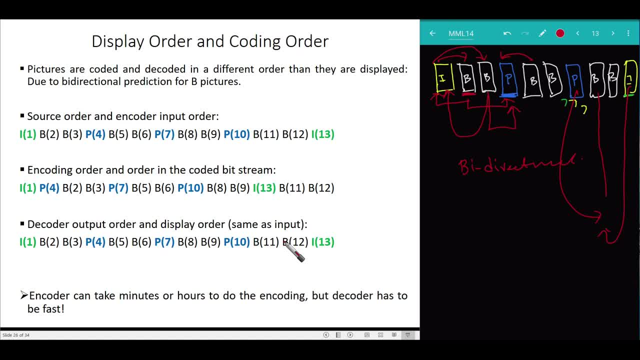 Okay, But think about that. I mean definitely. you know, when we see, you know, our encoder, There is some differences. Let's say: this is our encoder, This is our encoder, MPEG encoder. So the order in which we are, you know, supplying the you know video. 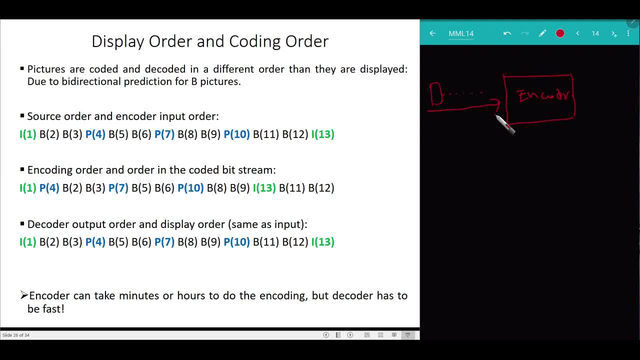 For example, this is one frame- second frame, second frame- But this output order is very different. Why? Because you know, for example- let's think about that- you know we have a frame Frame 1,, 2,, 3,, 4,, 5,, 6, 7.. 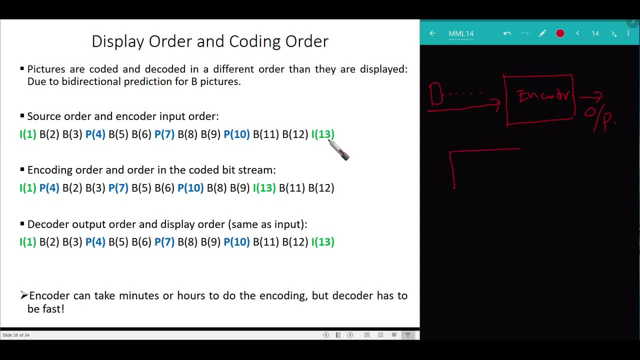 Up to 13.. Okay, So we have a video. We have a video of 13 frames. Frame 1 to frame 13.. Okay, Frame 1 to frame 13.. So this is that one, But we will consider this one as an I-frame. 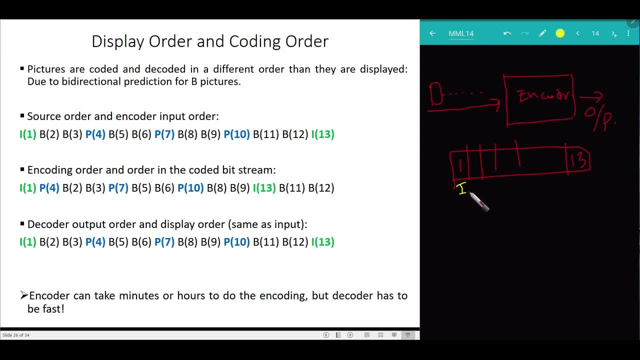 Right, Okay, If we consider this one as I-frame and let's say, if we consider you know, this one next to is, let's say, you know, B-frame. So, and the next one, This one is P-frame and the next two is B-frame and the next is P-frame and the next two is: 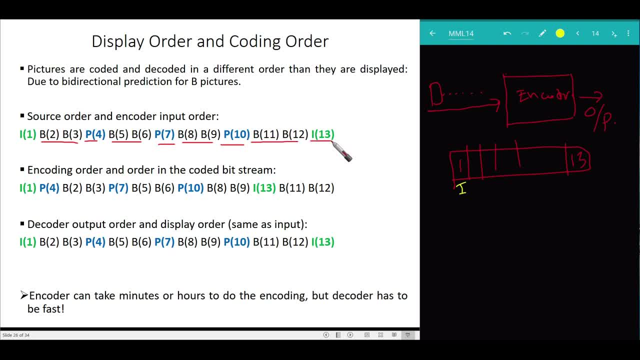 B-frame and the next one is P-frame and the next two is B-frame and the next one is again I-frame. If you think, if we designate our frame in this way Now, what will be the encode output? So definitely the very first things it should come is: it should come is definitely the 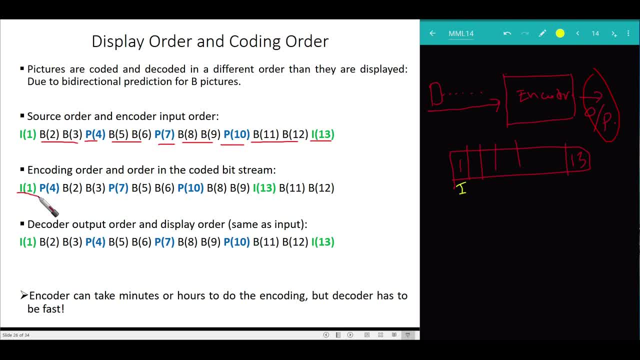 you know, the encoder output will be: the very first one is I-frame, But the next one will be P-frame. Because This P-frame? Because we cannot, we don't know this B-frame, We cannot, you know, generate this, you know B-frame without this P-frame. 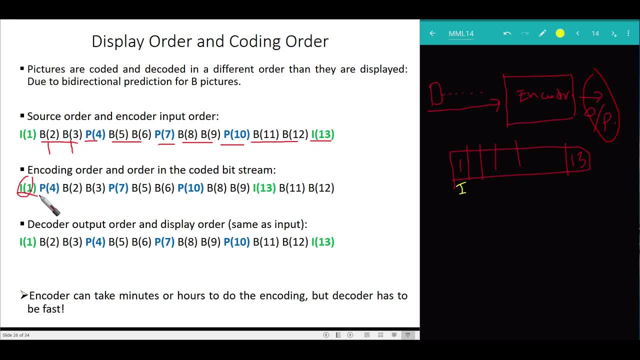 So that's why you know, this is independent. After that we constitute, we construct this P-frame, And then we constitute B-t and B-3.. After that we constitute, you know, P-7.. And then we have B-5 and B-6.. 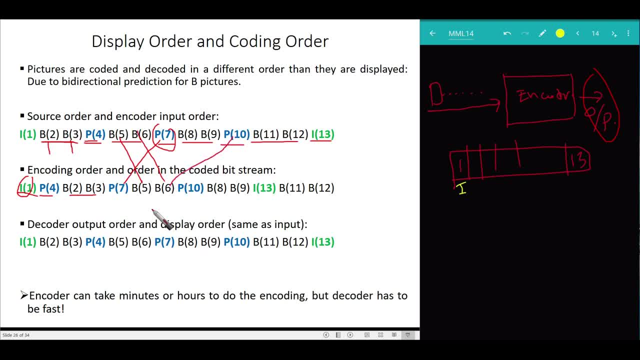 After that we construct, you know, you know this frame, And then you know, Sorry, this one, And then we construct this one and this one, So see, So the very first one is: this frame is I-frame. 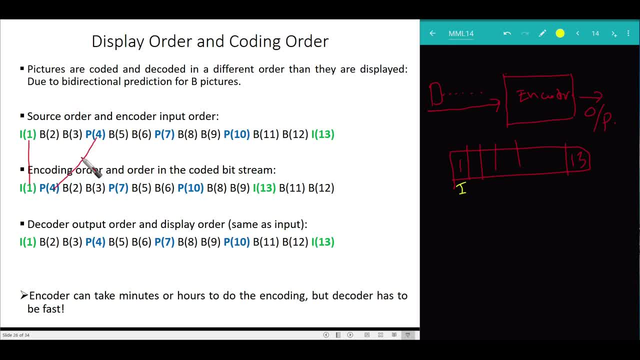 That's fine. And the next is P-frame, Because you know, because you know, to calculate this B-frame, we need this P-frame. So that's why the very first thing is this I-frame and then this P-frame. 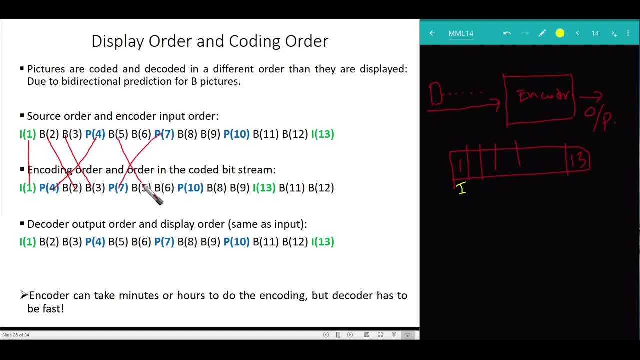 And then we have you know this, P-7. And then this one, And then this one, And then we have this one, And then we have this one, And then B-9.. And then 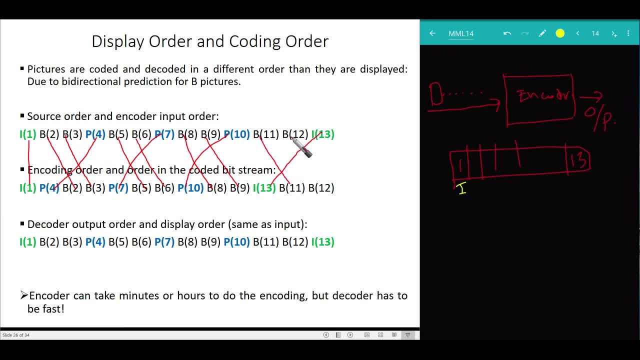 And then this I-frame we should have, And then this one, And then this one. So the order of the original image is basically changed as the output of the encoder. So this is the output of the encoder. 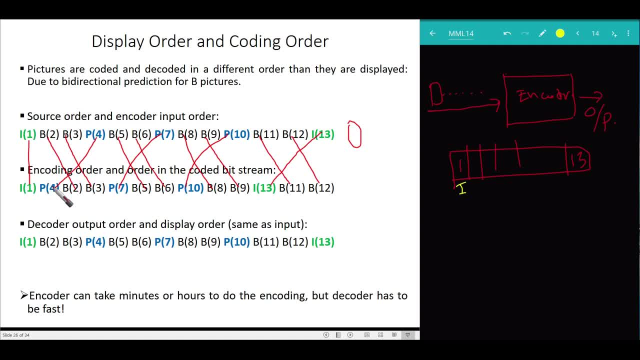 The order of the encoder is like this, So it was 1,, 4,, 2,, 3, 7, you know 5,, 6,, 10 in this way, But definitely the display order. when we decode we will get return back to our original order. 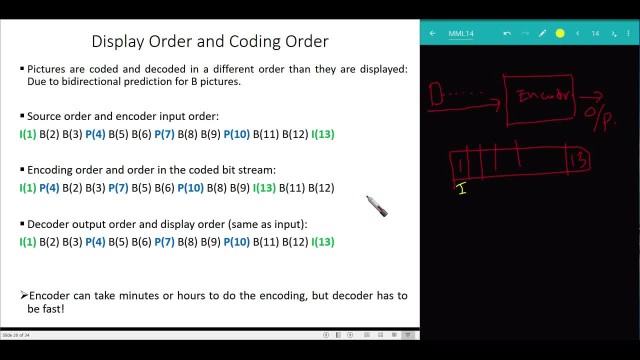 Otherwise the display will be very different. Okay, So that's why you know encoder, you know to calculate this kind of you know frames and ordering, reordering the encoder sometimes take you know minutes or hours to do the 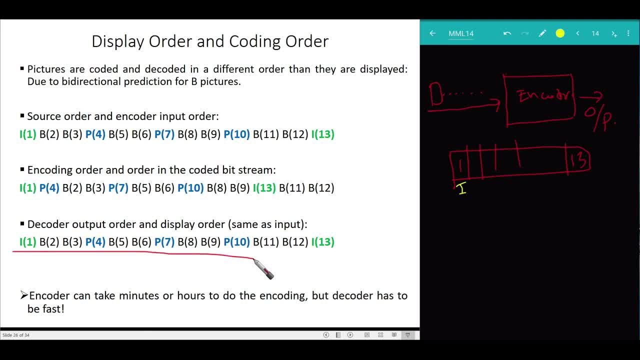 encoding, But decoder definitely needs to be fast because you know when we look at the video we can't wait for, you know, to calculate the video or those kind of things. Now think I mean this. actually the magic thing is this. 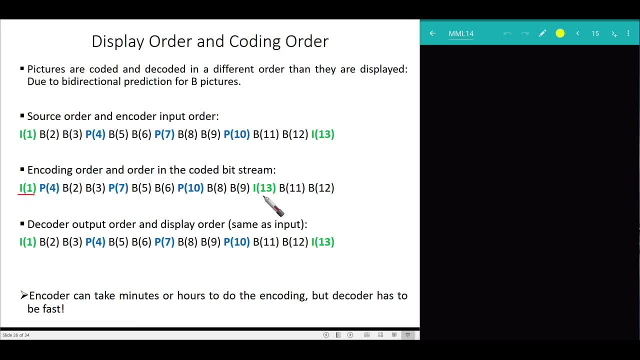 This iframe. If this iframe is missing, for example, let's say this iframe is suddenly missing, So that means what? If we miss this iframe, maybe you know, some very strange picture will become, because we don't keep the track of the iframe anymore, and some very, you know, peculiar, you know. 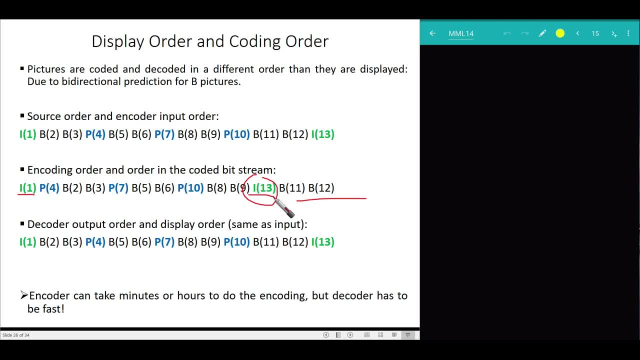 some another kind of strange reference frame might be coming And if we have the different, you know reference, you know frame, definitely the subsequent pictures will be different. So, again, we know we need iframes, Iframe, and we have to wait until the- you know, the correct reference frames comes. 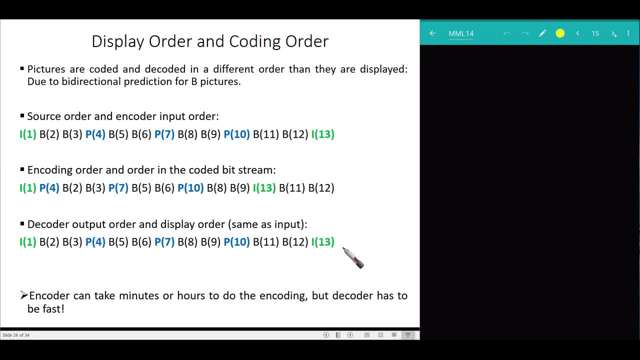 So sometimes when you look at the video- sometimes we can see that video- suddenly you know some very peculiar, you know some frames comes, And then again, after some times you know it, it, it, it again become OK. 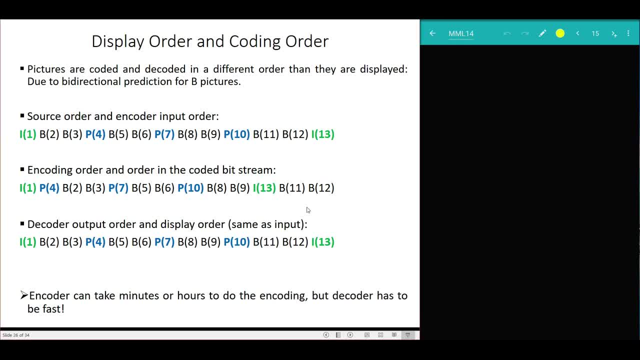 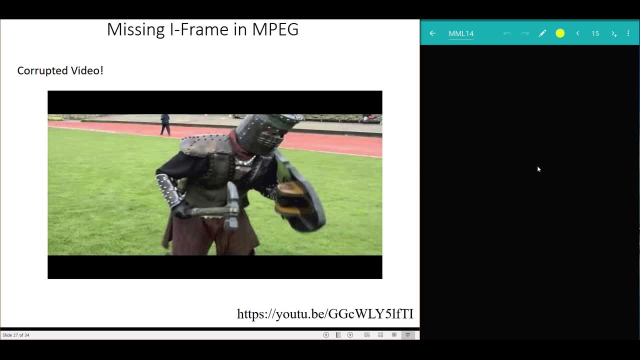 Right, So so what happens? I mean, if you- if you really you know- miss some iframe that how this video looks like? you know, see, you know, here I have it. You know, very small video clips for you and I will play. 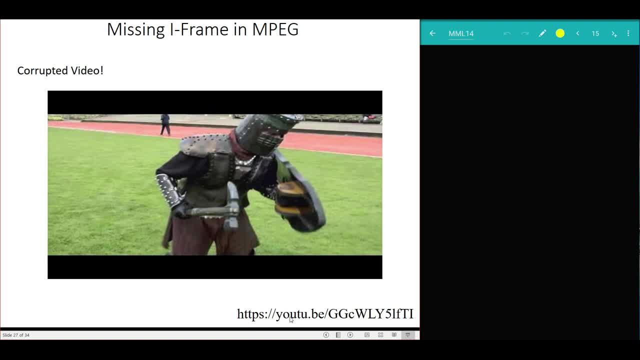 You can also look at. you know this video. you know this video one. You can see this one, this Lee and there, you can see this. you know video, So I'm not sure that I'm just waiting just just for a second that to see this one is coming or not. 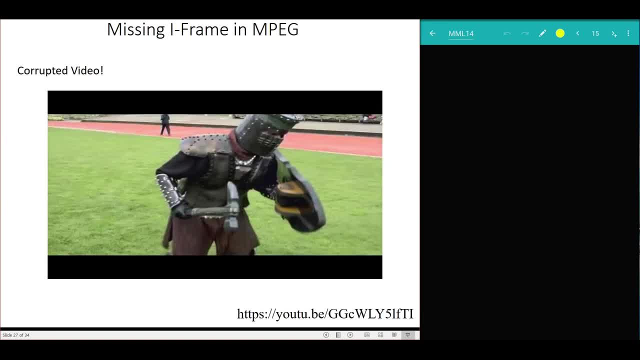 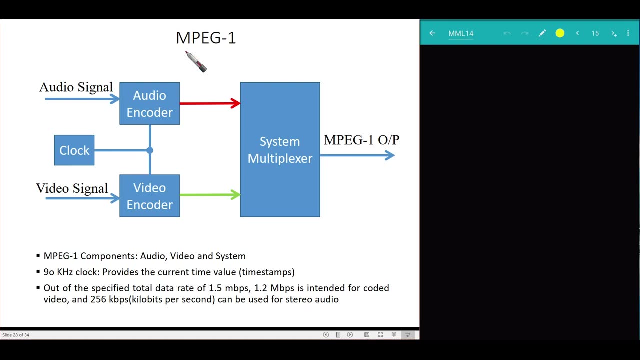 So actually it's not coming here so you can just go and check That what happens, you know if missing iframes you know occurs. OK, So MPEG-1, you know, when you look at the system perspectives, you know how it works- is like this one that you know we have an audio signal and we have video signal. 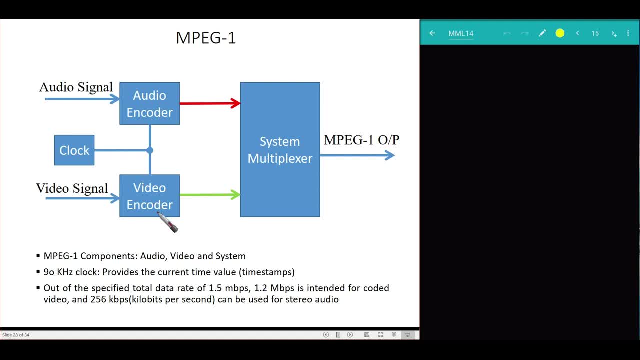 The audio signal goes to the audio encoder. video signal goes to the video encoder to maintain the. you know, you know time, to maintain the time So we have to have time stampings and for that we need a clock. So this clock is kind of, you know, 90 kilohertz. you know clock signals that maintain the time stampings and synchronizations. 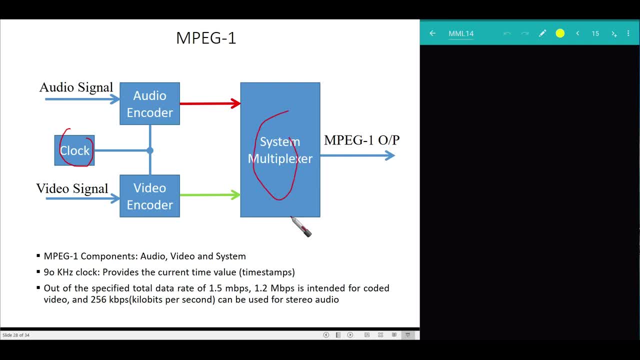 And there is a multiplexer, you know, based on our timing and sequences and algorithms, it just, you know, mix up this audio and video And then, finally, the stream of this MPEG, you know video, comes up here. This is the output signal. 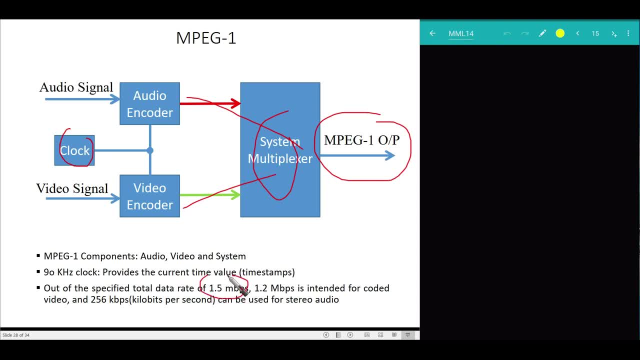 So generally, you know, 1.5 Mbps is the typical data rate in MPEG-1.. So out of out of it, you know, 1.2 Mbps is basically introduced for coded video and 256 kbps for stereo video. 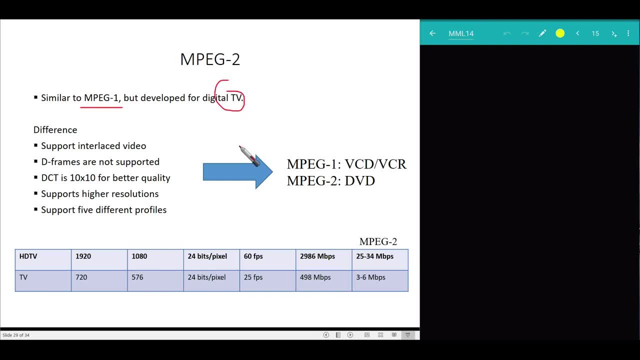 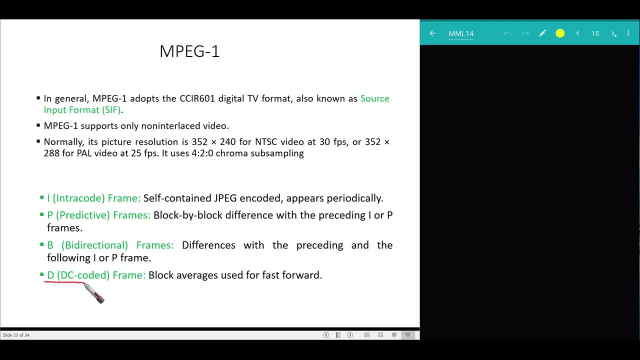 MPEG-2 is similar to MPEG-1, but it developed for digital TV. The difference is, you know, it's supported interlaced video and D frames are not supported And if you see That, you know we mentioned that in MPEG. you know there are other kinds of frames called, you know, D frame or DC frames. 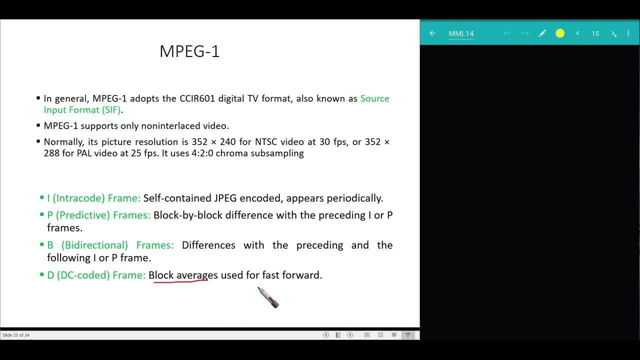 This is used basically for block everases when we do some fast forwarding. So at that time we need that kind of things. and P frame- predictive frame- is block by block differences with the preceding I frame or P frames. OK, so P frame, you know P frame is. 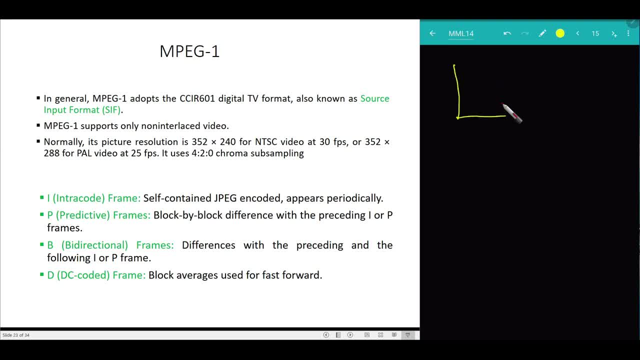 Let's say if it is a P frame, so it means this frame is kind of you know. let's say what is the differences between these block, So not pixel by pixel, that what is the difference in this block and this block? 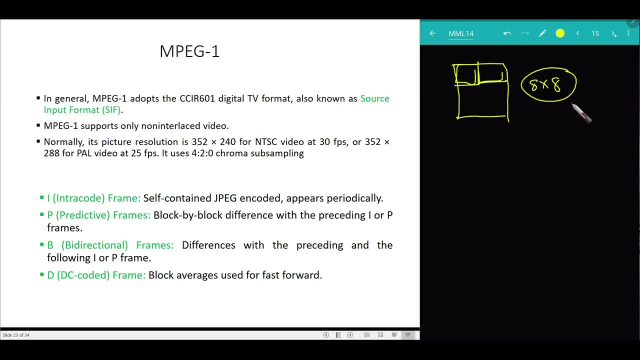 So this block size is eight by eight block size, So from one frame to another frame. So that's why it is a block. by block differences and bidirectional differences is differences between simple I frame or P frame. I explained before. So the block size in MPEG-1 is eight. 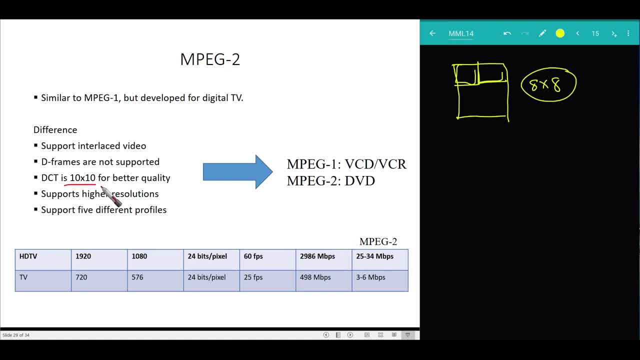 It's eight by eight, but in MPEG-2, the block size is ten by ten And it also supports higher resolution and it has different kind of, you know, profile. profile means you know what kind of data rate, what kind of frame rates, different kinds of combinations. you know this MPEG-2 supports. 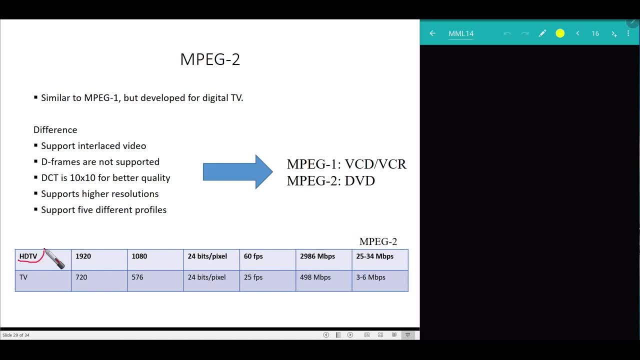 So, for example, let's say- here is an example- let's say HDTV. you can consider the high definition TV. The resolution is, let's say, 1920 to 1080 and 20.. Four beats per pixels. 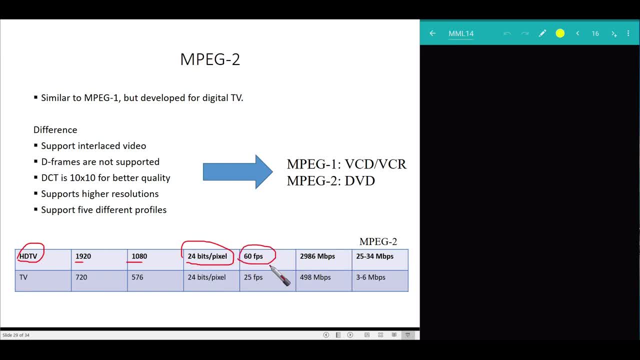 You know, and if we have 60 frames per second, so if you calculate the data rate, it will be uncompressed data rate will be 2986,. you know Mbps and you know that, how to calculate. you know this one right. 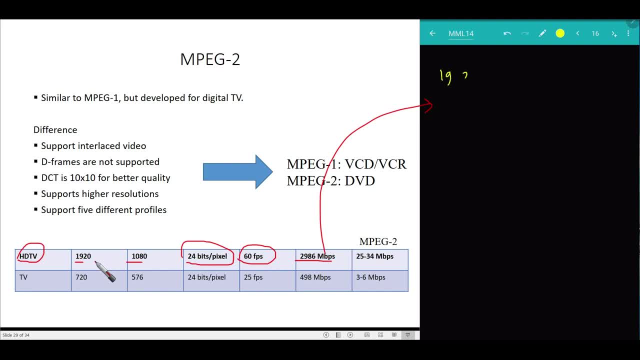 So, for example, 1920 multiplied by 1080.. This is one single frame size And for ESP, so that means that means this number of pixels. for ESP pixels, we allocate 24 beats. you know, to represent the data, maybe color, or maybe whatever. it seems to RGB color. 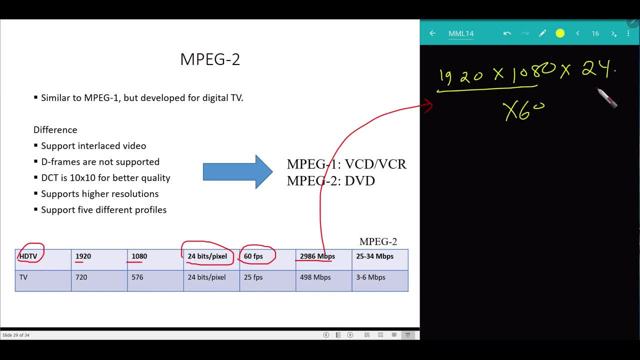 And we have, you know, 60 frames per second. So if we just, you know, multiply these ones, so it will be kind of approximately 2986.. Mbps. can check it at home. But if we do the MPEG, you know, compression, MPEG-2 compression, then the compressed video side will be around 25 to 34 Mbps. 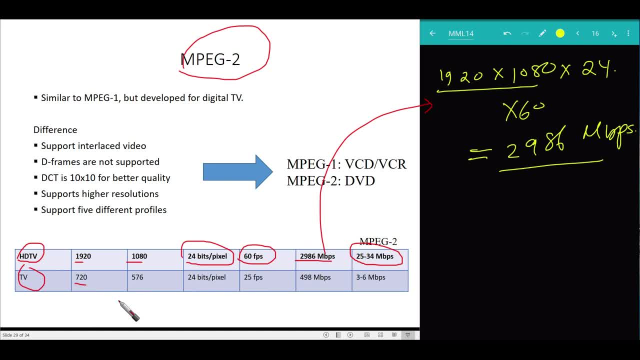 For television signals we have, you know simple: 720 by 576.. So what does it mean Actually? 720 by 576 or 1920 by 1080.. If you remember, this means that: how many pixels? How many pixels are there horizontally and how many pixels are there vertically? 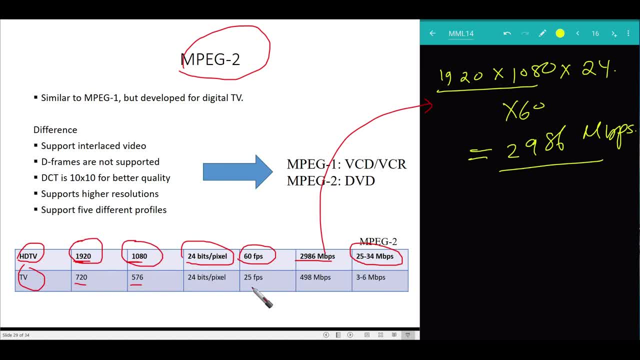 That means this is image height and this is image width. Okay, So ultimately this TV signal is text. you know, if you don't compress there's around 498 Mbps, But if you compress then it becomes 3 to 6 Mbps. 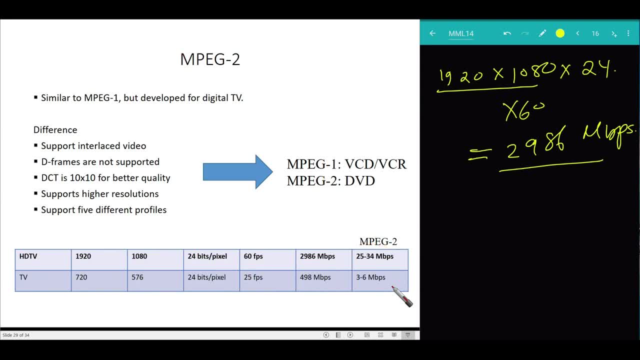 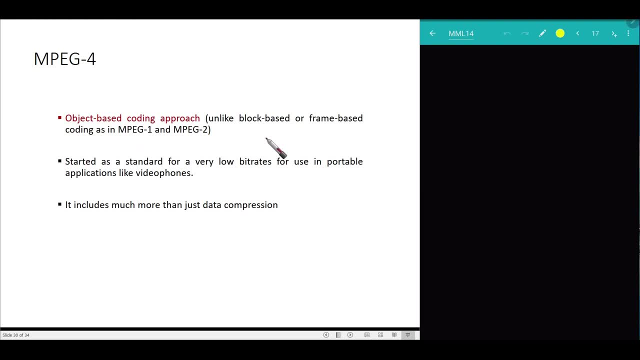 So you see that the power of MPEG-2 compression Now MPEG-4 is basically, you know, it's not block based or frame, It is frame based coding like MPEG-1 and MPEG-2.. It is kind of, you know, object based coding approach. 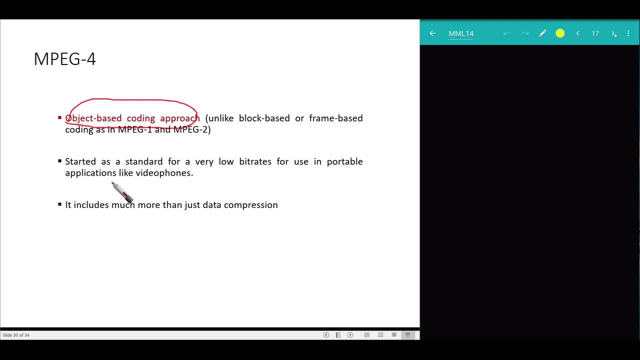 So object based coding means from the frame we detect the object and then we manipulate that object so that we say content based manipulation. It basically started, you know, for the applications of, you know, portable applications, like, you know, video phones. 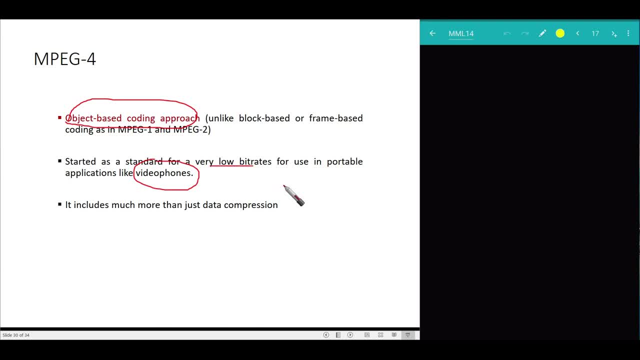 And are originally targeted for video phones for low bitrate applications. so I would say that you know MPEG-4 is not really data compression, it's actually much more than that. you know, for examples, think about here this kind of you know MPEG-4. you know many manipulations and 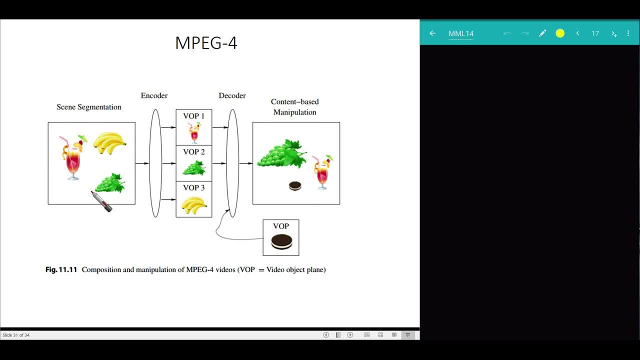 processing, for example. let's say, here is a scene segmentation. we just, let's say, we did some sort of you know, segmented things and we have, let's say, banana and here a grab and some juice, and what you do is kind of let's say, we just transmit. 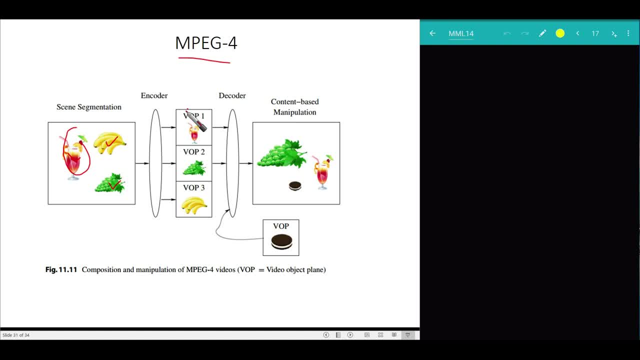 to MPEG encoder and let's say for this one, this is separate. you know we can say separate plane video plane and object plane, video, object plane. let's say for the grab, and then you have the banana, like this one right now, what we can do, and let's say some sort of content based manipulations, for examples. you know, let's. 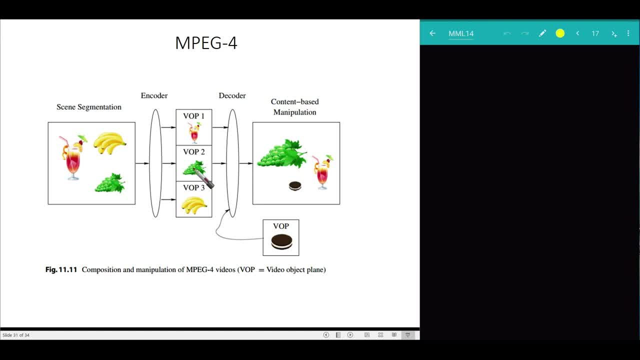 say we keep this object as it is, and, and for this object we just enlarge, and and for this object we just delete, and, and then this object we can insert. so this sort of in, and you see the output is kind of content based manipulations. so this can be done in MPEG-4. so there are some other kind of you know, 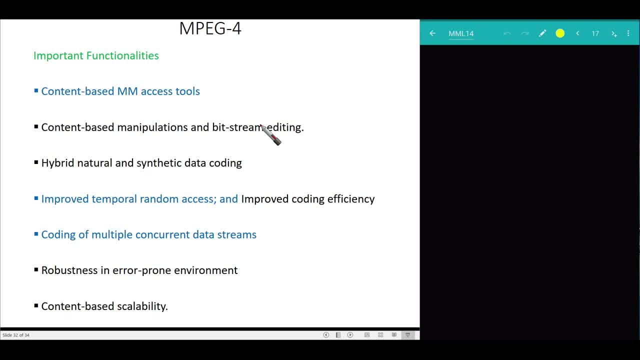 functionalities. the very most important functionalities that we can see in MPEG-4 is kind of this: you know, content based multimedia access tools and and some other kind of- I don't know, maybe, maybe, maybe temporal random access you can. you know, access in anywhere and coding efficiency improved also some more. you know robust. 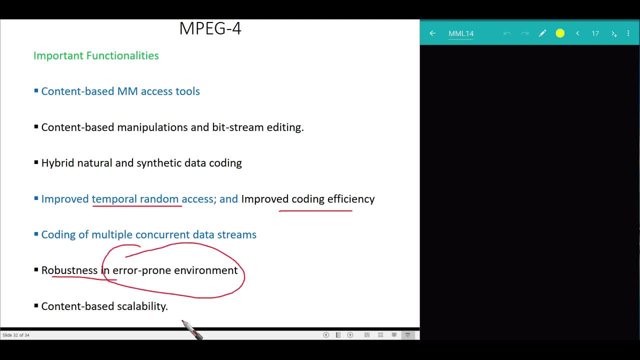 to errors. that means less error happen. if even though you just communicate in a very harsh environment is still you know it can communicate well and it's callability, so you can, you know, try to search what this means at home and see that to sharpen your understanding or more. but I just gave you an. 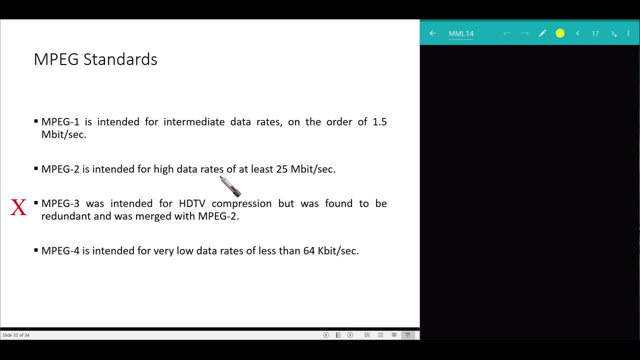 basic idea. so overall the MPEG standards is: MPEG-1 is for intermediate data rates and you know it was for 1.5 Mbps or something. MPEG-2 for high data rate applications, for example around 25 Mbps, now MPEG-3. there was MPEG-3 for HDTV compression, but later on it was March to MPEG-2 and MPEG-4, as I 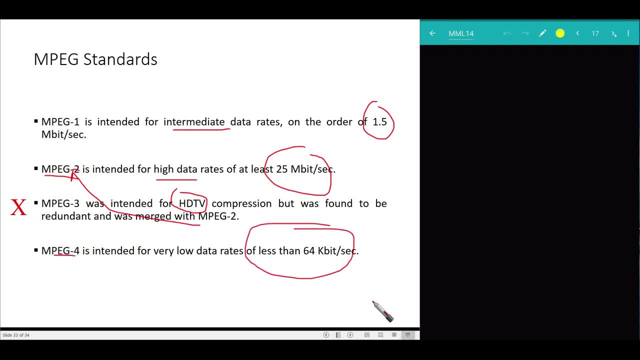 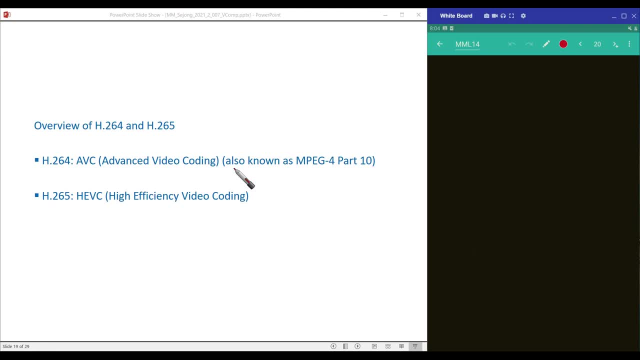 explained, usually for low data rate applications, for examples around 64 kbps. okay, now let's talk something on this: H.264 and H.265- and as I said in the beginning that this is somehow we considered an advanced as advanced video coding, and also this one is very. 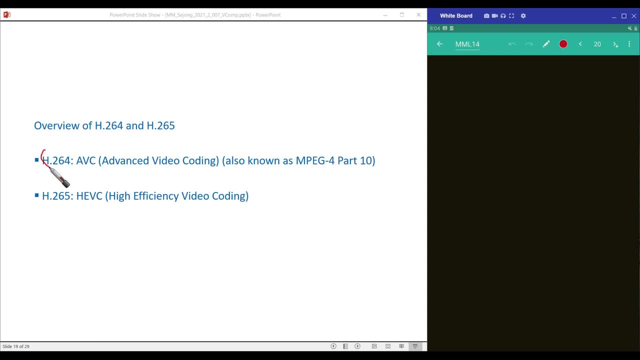 advanced, that is, high-efficiency video coding. so this one is started, you know, firstly, maybe around 2003-2004 and if the latest version is, you know, 2019, and this one started around 2013 or 14 and its latest version is also 2019. so these are very useful, especially this. 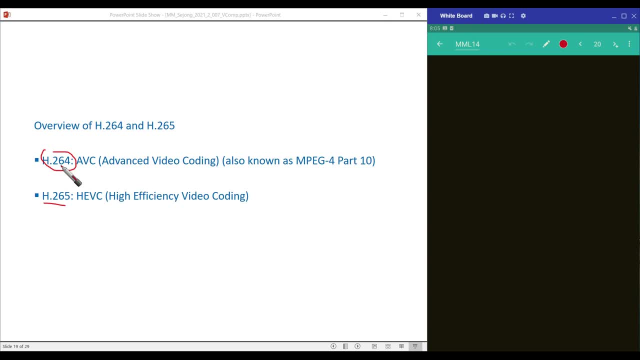 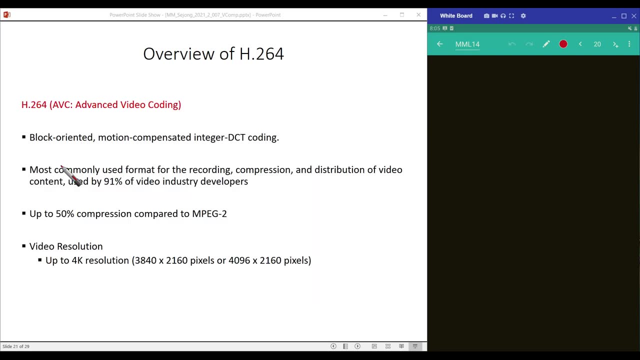 you know H.264 is still being used, you know, by by many of the software's and companies industry. so we'll be coming here. but let's see, you know some features or some features that are still being used by many of the companies industry. so we'll be coming here. but let's see, you know, some features or some. 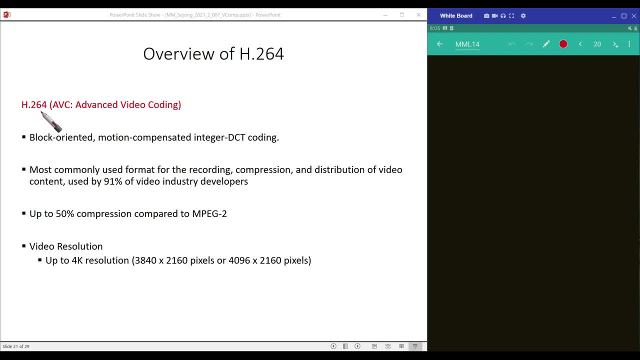 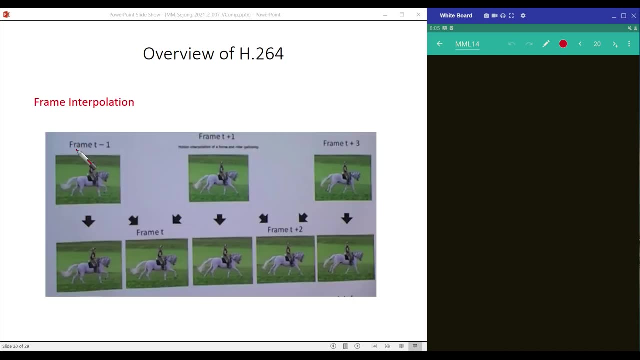 description- general descriptions on H.264. this is basically a block oriented. you know motion compensated integer DCT coding and you know what is block oriented? it means it's simply block by block. and so what is this? let's I talk that. you already know that how frame interpolation works, so that is you know. 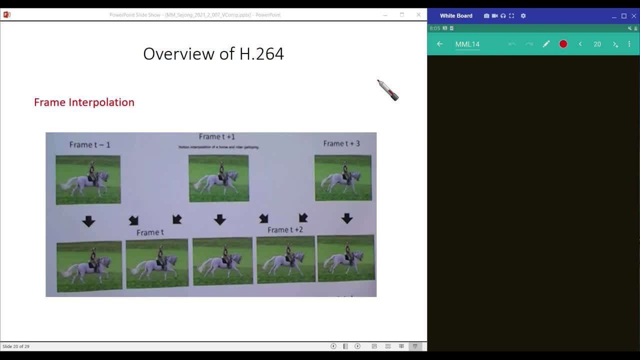 for examples. let's say: you know, the video is basically the sequence of frames, right? let's say this is a frame interpolation. so let's say this is a frame at T minus 1, at T minus 1 time in stand, and this is the next frame at T. 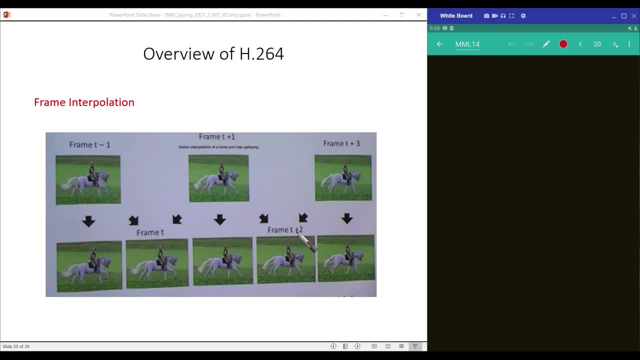 and this is the next frame, T plus 1, this is the next frame T plus 2, this is the. you know some consecutive frames right and, as you well, as you already know that we don't send all the frames right for examples, you know, let's say, we send this. 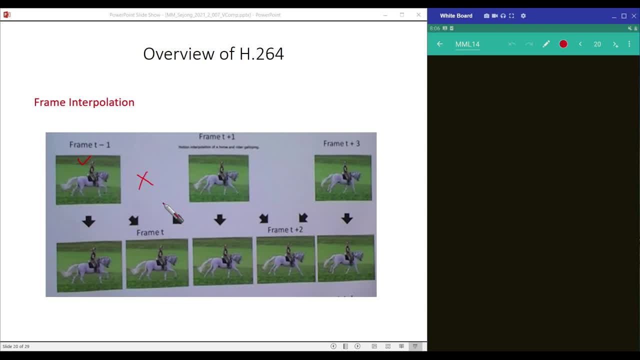 frame and we don't send the next frame. and then let's say, we send next frame and we don't send the next frame and we send the next frame right and in the receiver side, what we do, basically we use, you know, this frame and this frame to generate this frame right. so this is calling a frame interpolation. 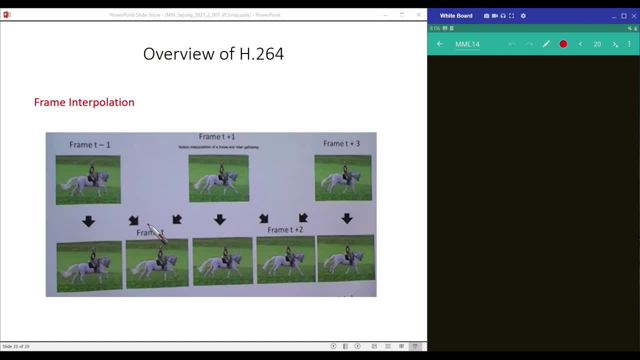 that the missing frame- not only the missing frames, I mean the frame that we didn't send. or we can consider that this one as I frame and and then maybe this one is a P frame. so, using I frame and P frame, we constitute or we recover the. 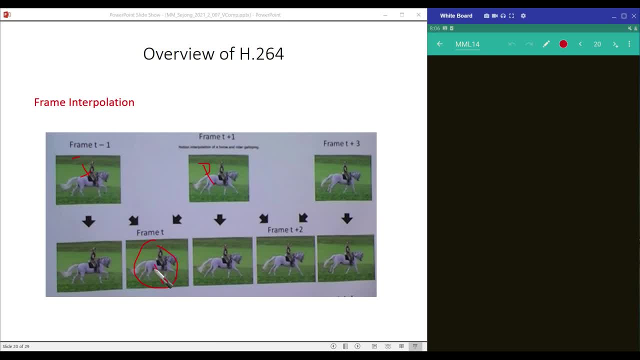 frame. I know, maybe B frame. we say maybe B frame, right, as you know this. So and how we do that, I told you this is some techniques called motion compensation, because it we see that how the object or you 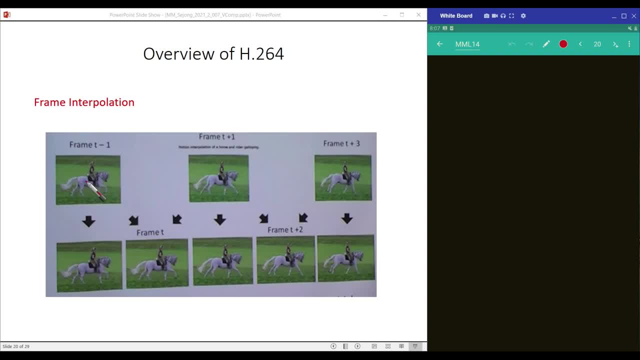 know, some point is basically, you know, moving towards a particular directions. For example, in this scenario, we can see that this object, or, let's say, this picture itself, is moving towards these directions, or whatever it is. So if we just, you know, see this one and this one, then 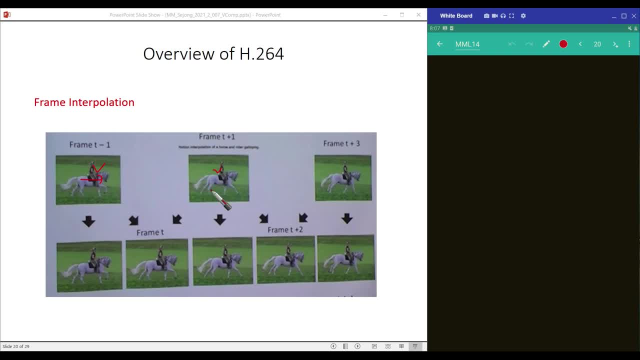 you know we can estimate the motion of this object and accordingly, you know we will generate, you know this object. So based on this is we say that I mean technique is motion compensation technique. Of course we are not studying how the motion compensation technique itself works. 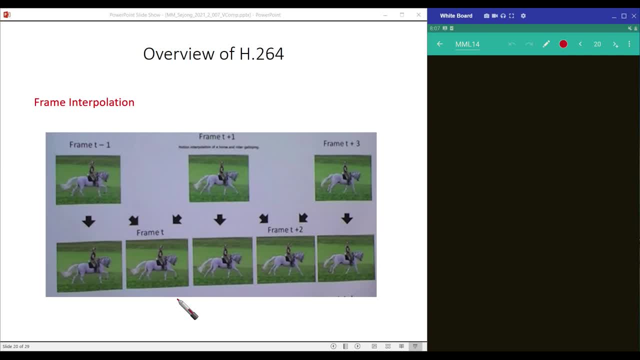 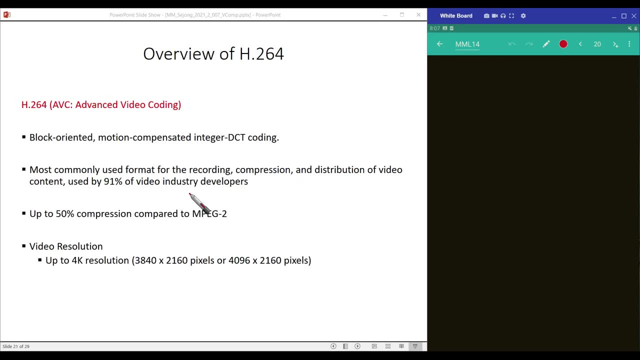 So that is a different. you know things For our multimedia stuff, you know we don't we don't need to know those things, We just know that you know we use motion compensation to generate this one. So this is basically you know. we say you know frame interpolation, That. 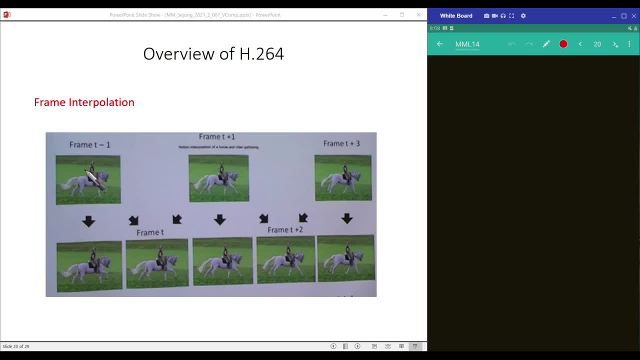 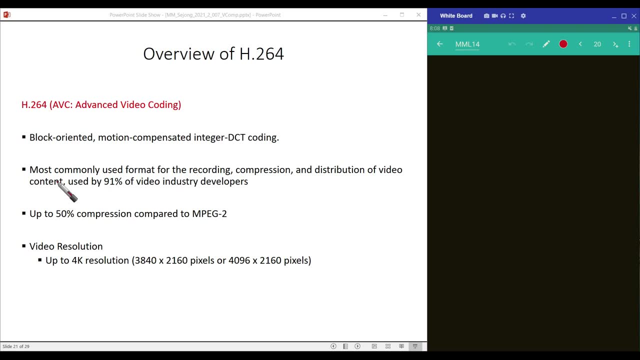 means you know, one frame to another frame, or maybe from I frame you know to next B frame, how we generate those And, as I said, that is basically mostly commonly used format for the recording, compensation and distribution of the video content And you know, typically you know. 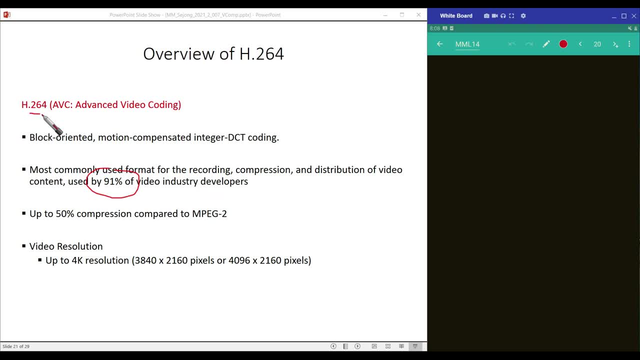 more than a hundred percent of the time. we don't need to know those things, So we just know that. you know 90% video industrial developers they use. you know this AVC technique And compared to MPEG-2, it basically achieves 50% compression. It's also provide the resolution up to 4K, So you 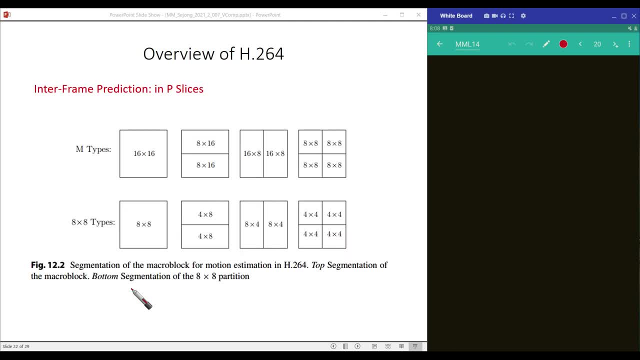 know these things. I explained in details. So when you do this, you know frame interpolations, for examples, you know using I frame and let's say we like to generate. you know, let's say P frame something. Okay, We say P slice sometimes here. 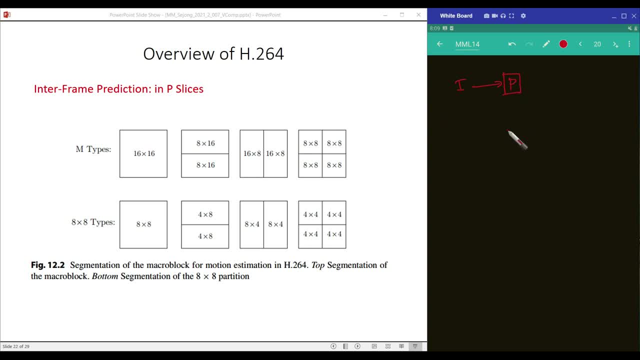 And I will see that what is mean by slice a little later in H.265 concepts. But let's say, you know, for this time being it's somehow another you know frame or something. Anyway, so this there are. you know, two types of blocks we use here in this H.264.. One is 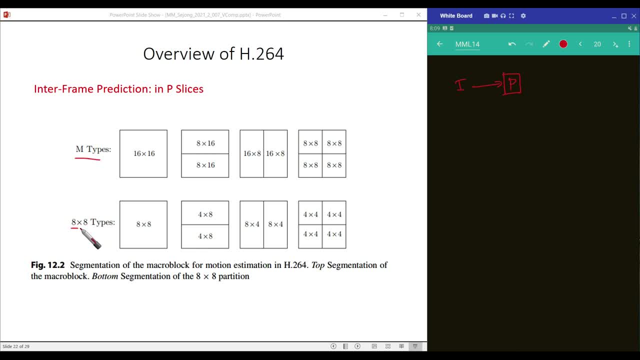 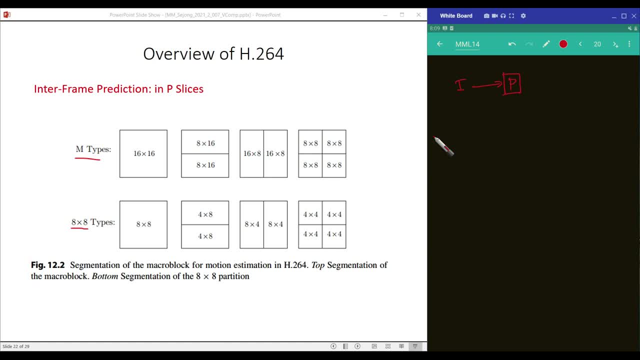 that will M type block. you know the block size, even it might be, you know, 16 by 16.. So so, for example, think about that in a particular frame, And you know the frame means we can. 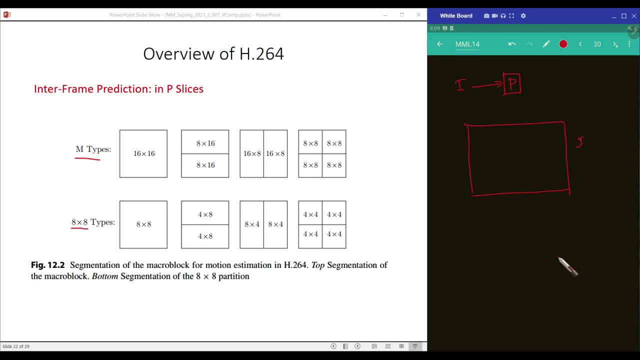 understand it is a JPEG frame or something. So let's say JPEG frame, JPEG image. So here maybe large area, maybe maybe let's say very large area, or maybe large in a very, you know, greater area, big area, maybe you know the similar. 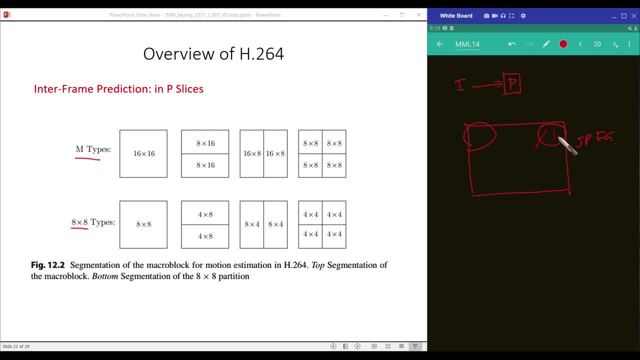 values are there, that means more smooth version, right, more smooth area. so at the time maybe if we know one pixel values, so maybe other pixel values are similar in that area. so in that kind of situations, you know we can use this large, you know values like 16 by 16, you know size. 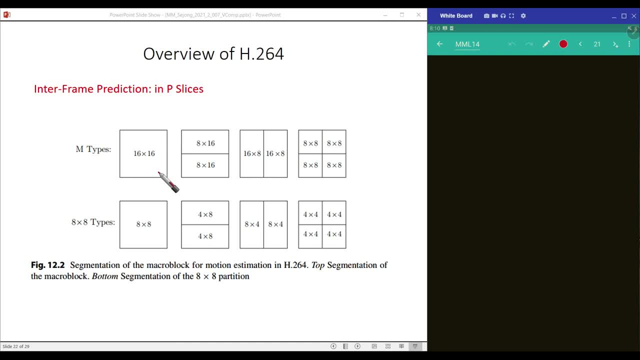 but definitely, you know this 16 by 16 block. we can, you know, sometimes also divide some smaller parts. for example, we can consider 8 by 16, 8 by 16, so that means this 16 by 16. we can divide like in this way. this is vertical divisions. we can also like horizontal division, that means this one and 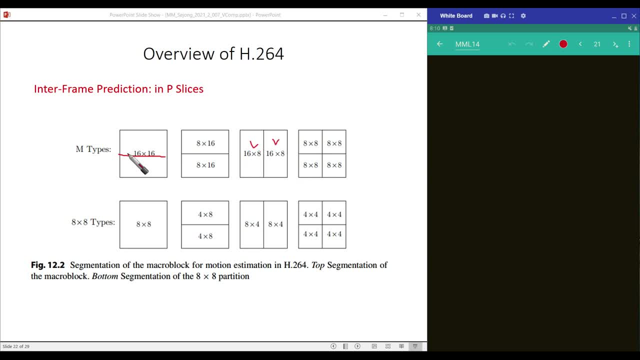 this one that is 16 by 8 and 16 by 8.. so this one is 16 pixels, you know, height, and 16 pixel width. so the 16 by 16 can be, you know, implemented in, you know, 8 by 16 and 8 by 16, in this configuration, or in this configuration, or. 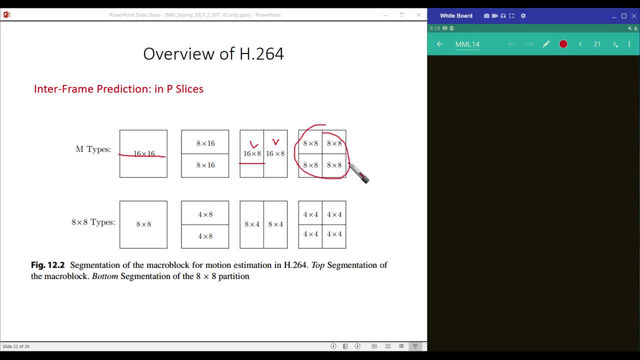 maybe four, 8 by 8 configurations. so, whatever it is, it is some sort of, you know, segmentations of macro block while we do the motion compensation. so, for example, since that that's, we have the big image. so what we do, each block, let's say this is a block, right. 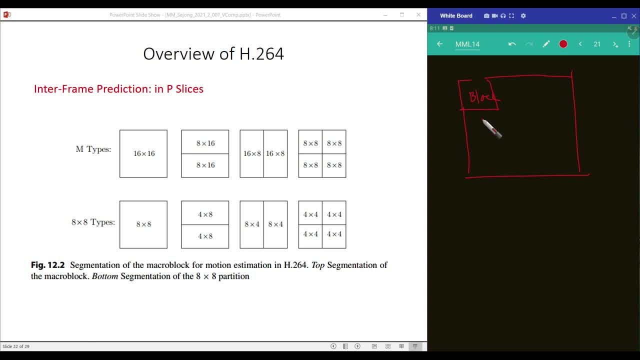 8 by 8 or 16 by 16.. so we'll see that. what is the situation in this block and what is the situation in the next frame in this block? okay, in the next from this 8 by 8 block. so we try to see the. 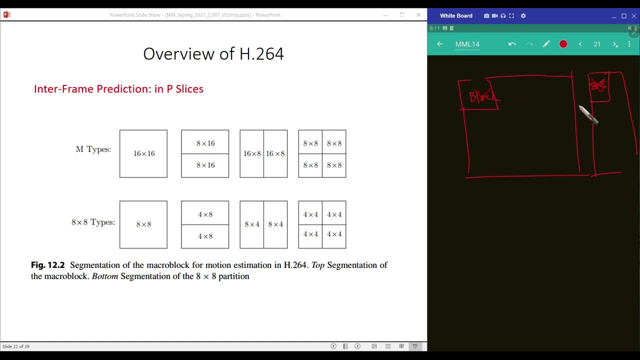 differences between this block and this block. in this way, block by block, we do this motion compensation, so whatever, and then if the image somewhere is, you know, maybe many changes happen or maybe very details we like to capture. so at the time our block size should be smaller, so we 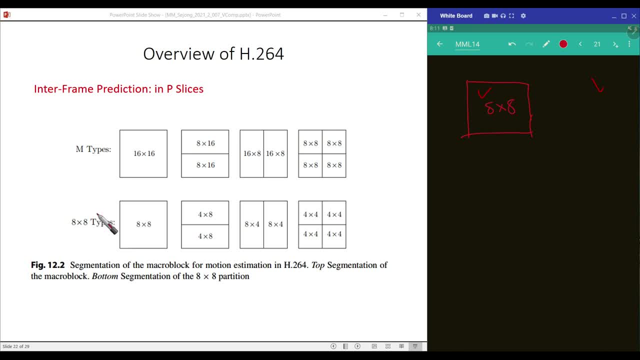 can think of 8 by 8 block size And that 8x8 block size event can be implemented in different- you know- configurations, For example, maybe 4x8, 4x8, or 4x8, 4x4.. 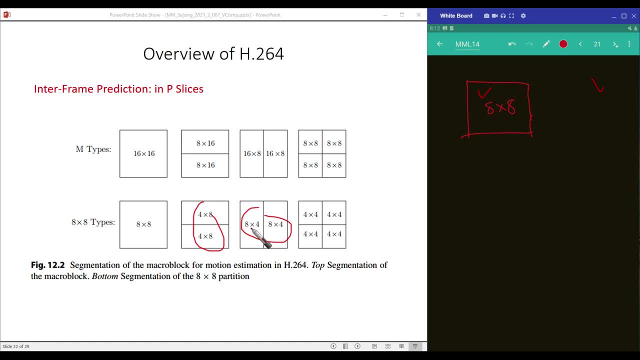 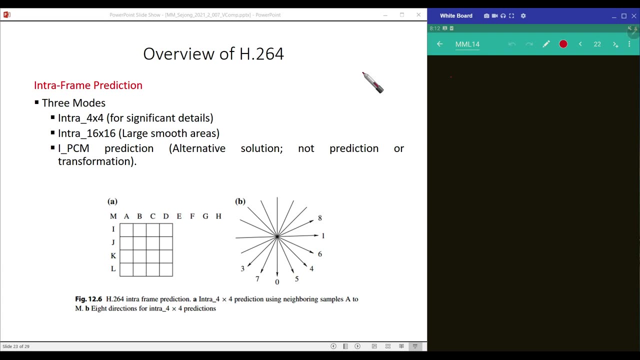 There are two 8x4, right, Or two 4x8. Or four 4x4.. This kind of segmentation we do, Or we can say partition. Now, this is, you know, a little different things, But think about that. we are sending, let's say, a particular frame, okay. 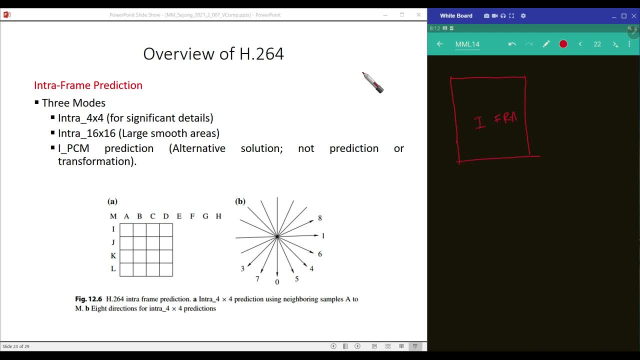 Let's say maybe I-frame itself, okay, Or P-frame itself, whatever it is, Let's say I-frame itself generally. Now, this frame, we can think that this is basically a JPEG image, right, And when we send an I-frame, definitely, you know, this is very important. 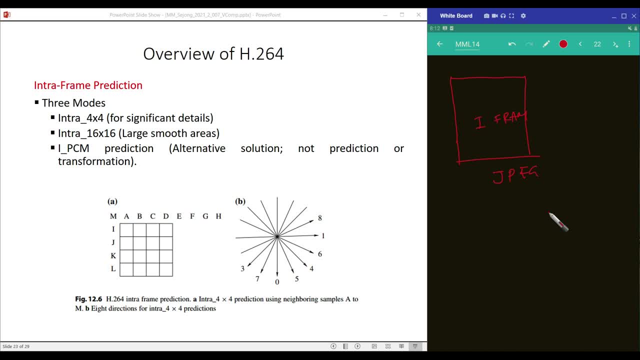 Because, based on this frame, the other frames will be generated. We can, you know, roughly, you know, say These kind of things Now, even within a single frame, we can actually, you know, compress our information And you know the JPEG how the compression done. 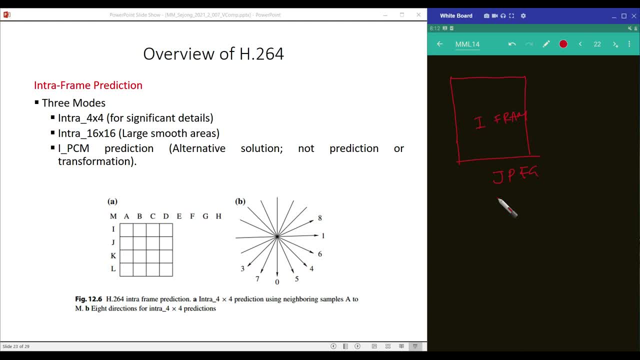 But forget about that JPEG. you know compression strategy. Even there are so many other strategies that actually this H.264, you know performed. So, for example, you know, think like that: Let's say: this is a 4x4, I mean a 4x4 block. 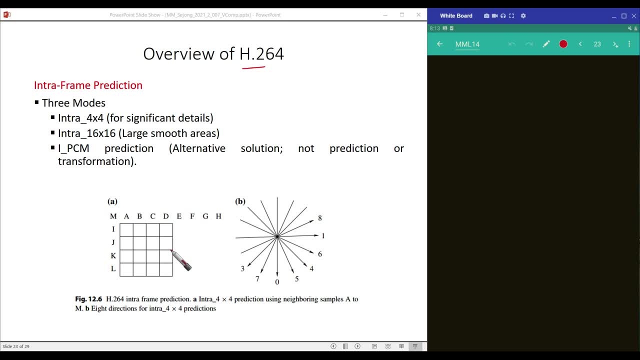 We can think that This is this 4x4 block coming from a you know big image. of course, you can think of Just a 4x4 block we are considering And let's say this is, you know? we can say that. let's say this is A, B, C, D, E, F, G, H, I, J, K, L, right. 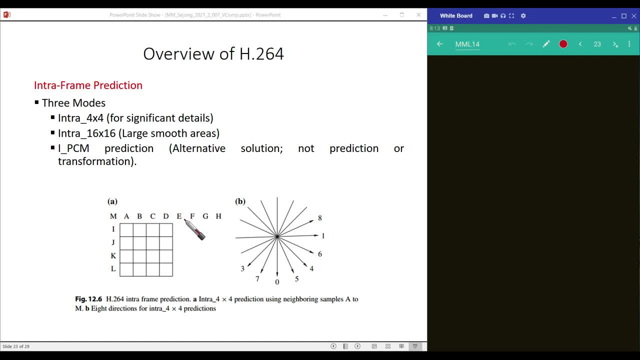 So we can designate, you know, the pixel level in this way. This is a 4x4 block. And then you know this one A, this one B, this one C, this one D and in this way H. 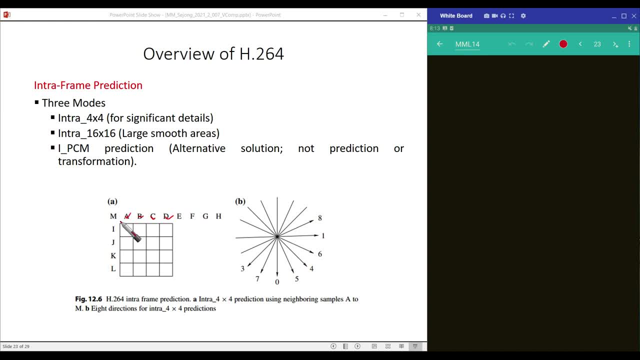 Right, And so these are basically the neighboring pixels, right? So that means you know this is a 4x4 block And this is, you know, another. you know, this is basically this: A is basically the neighboring pixel from a neighboring block, right? 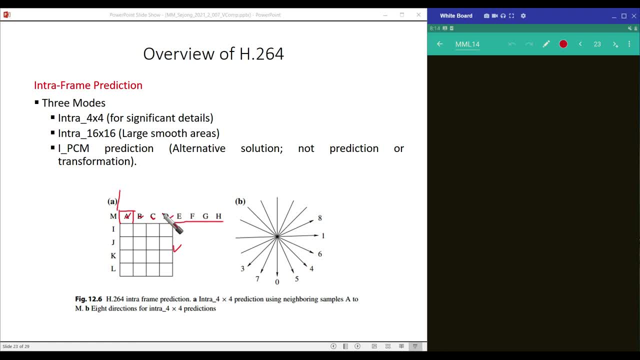 So this is basically a part of you know other block. We can think in this way: Now how we can actually compensate. See, maybe we can assume that maybe we don't need to send all of these pixels in 4x4.. 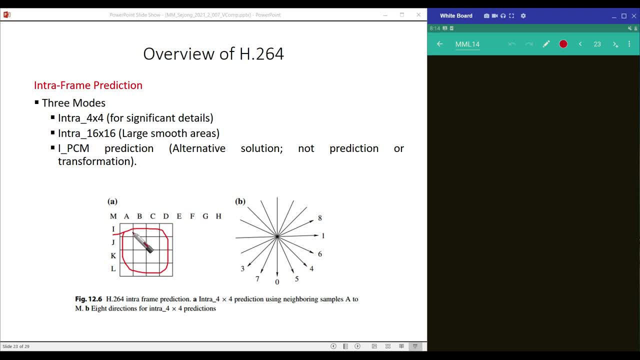 We can just copy the information, Rather what we can do. maybe we can copy the same A you know over the same you know here, right? Or maybe we can copy that: what is the pixel information in M pixels from this another block, maybe in this block? 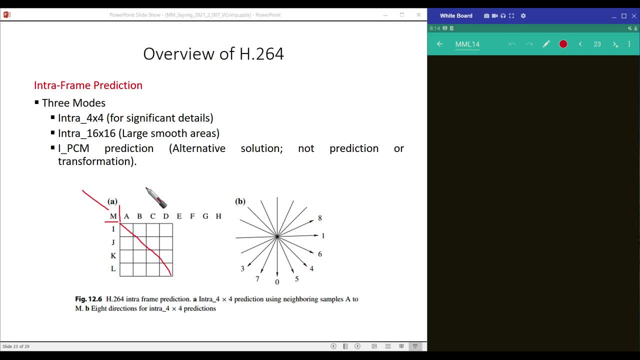 And these same values we can copy. So there are different kinds of. we say this is basically. we say you know the different modes, okay, We say different modes of prediction And these are the directs Corrections of those modes. 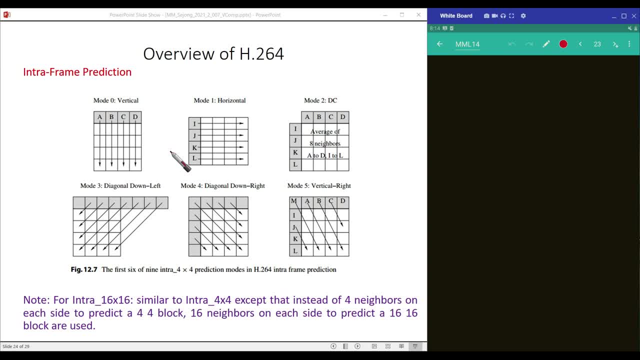 Let's say, we explain a little bit here. This is you know better, So we can use. you know. you know, here we are. you know there are actually, you know perhaps 9 modes, That is, mode 0 to mode 8.. 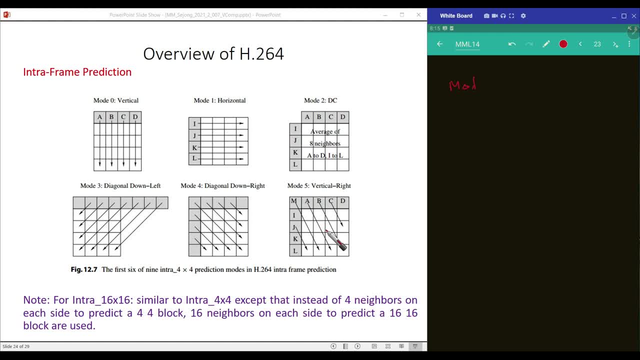 Mod. actually, you know mod right, You know it's called some mod 0 to mod 8.. And here some mods are. we are showing, let's say, vertical mod mod. that's mod 0.. 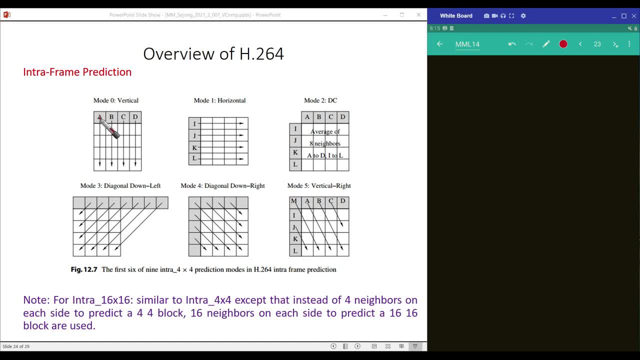 So it means that whatever the pixels A, we will just copy the same pixel values here, here, here and here. Similarly, the B pixel values will be used by the next. you know 4 pixels, Or you know we can use horizontal mode. 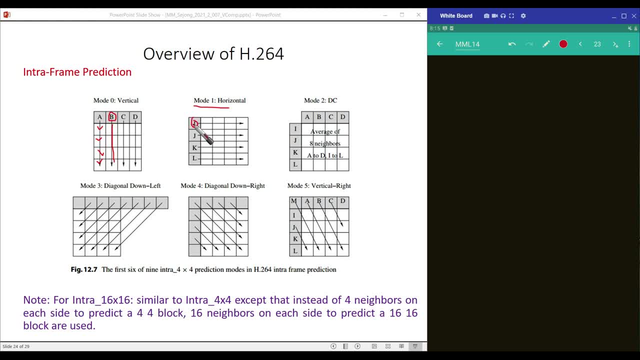 So, that is, we will copy the same values. that is, this is in ith pixel, j, k and l pixel, And these 4 pixels will be the same values as of i Or you know. we can Use, like you know, diagonal down left. 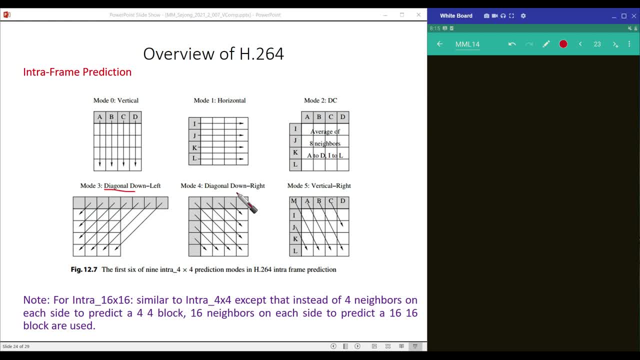 So this is diagonal going down and the left Diagonal down right Or vertical right. So there are different kinds of modes of predictions that we can use. So, for example, you know if I go here C. 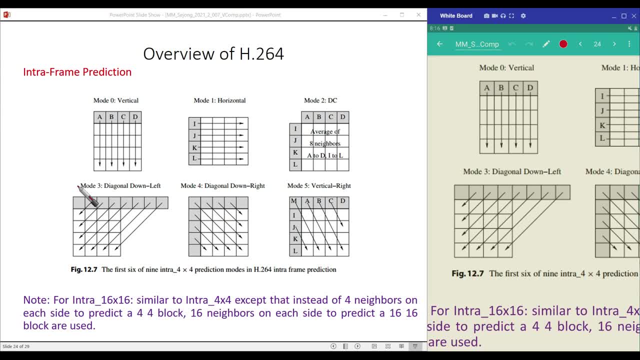 So what we are meaning? for example, let's say I'm just, you know, talking this mode 3.. So this is the same I just copied here. So this one it says: let's say, you know, this pixel's values is 5.. 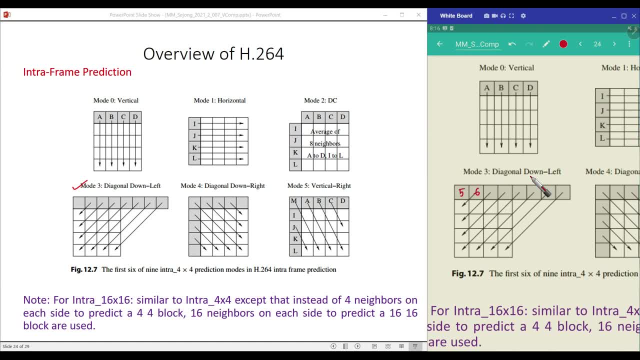 Okay, And let's say, this pixel values is 6.. This pixel values is, let's say, you know, maybe 10.. This pixel values may be 14.. This pixel values may be 46.. This value may be 5.. 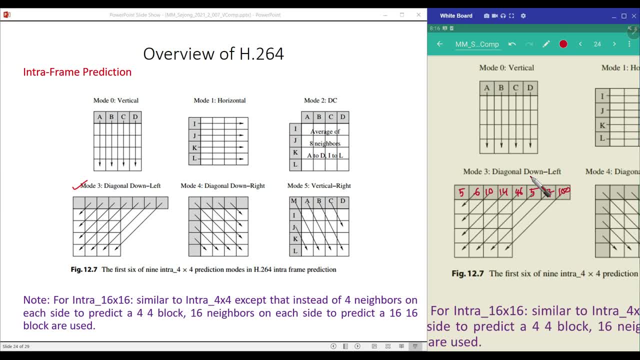 This is maybe 7.. This is, maybe you know, something like 100.. Okay, A very interesting thing is we can basically copy: See if we use diagonal down left mode. So that means you know these values will be 6.. 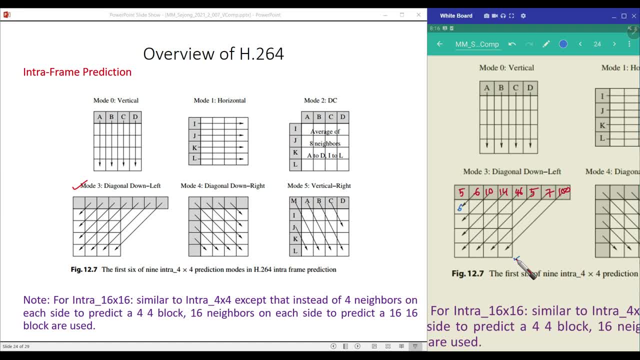 Okay, So this pixel, We are just, you know, talking about these 4 by 4 pixels here, 4 by 4, you know, block, This 4 by 4 block And this 6, basically copying from these pixel values. 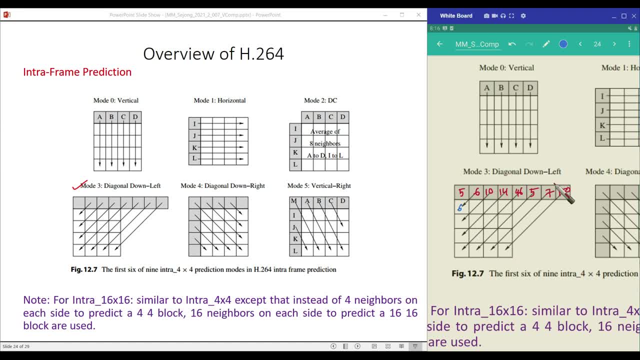 Right. If we add up this diagonal down left, And then you know, this 10 will be copied here and here. This 14 will be copied here, here, here. This 46 will be copied here, here, here, here. 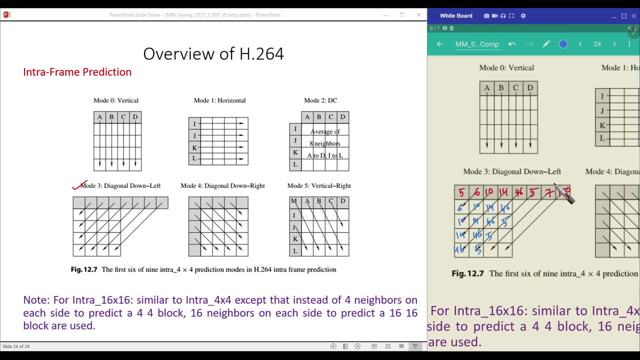 And this 5 will be copied here, here And here. This 7 will be copied here and here. This 100 will be copied just here. So you see, this is very easy. So once we have these, you know values. 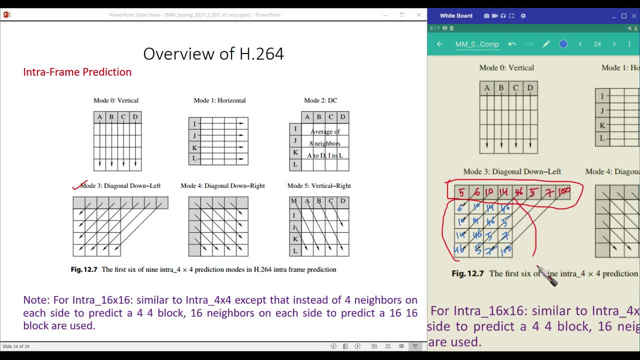 Then we automatically have you know these values. So what it means: We don't need to send this information, Just we only need to say that hey, we are using you know mode 3.. So this is one way that how, within a frame, we can basically compress our image a lot. 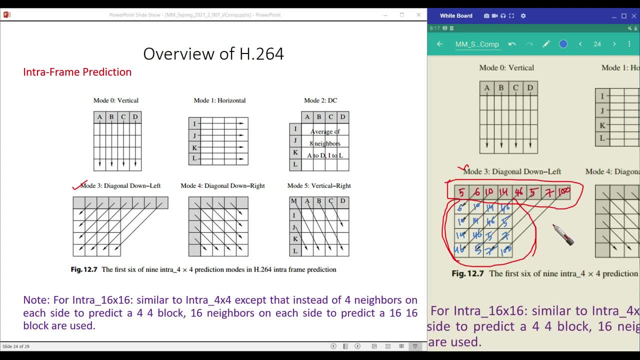 Because we are not sending this information. Rather, we will be copying these things, And it is you know in which mode will be used: Either horizontal mode or DC mode, or down right, vertical right or vertical mode. It depends on the algorithms or that how our human vision works, or depending on the natures of the 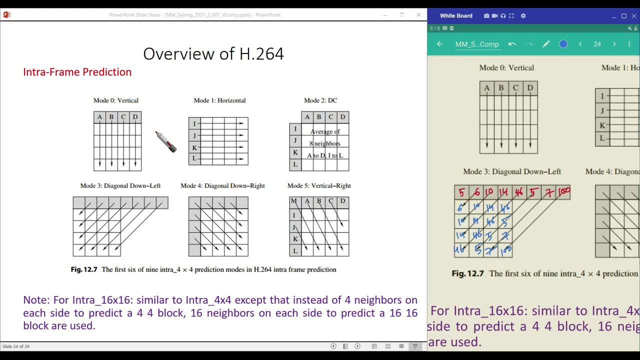 So that is a different things. So now I hope that you understand how this is called intra-frame prediction. That means within a single frame. when we are sending a single frame like this, You know, like a single frame, that this frame 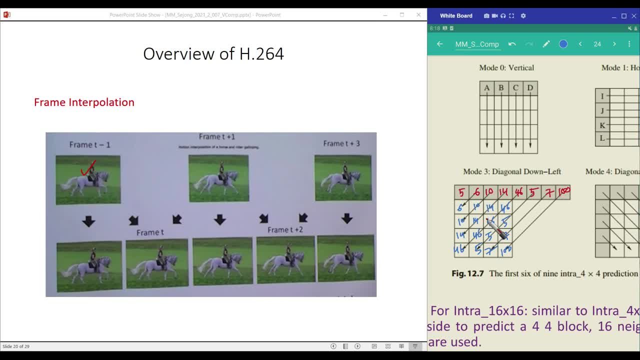 You know, within this frame we don't need to even send all this information, Right? Because in the receiver side we first generate this information using this kind of technique And then we also generate this information using its interpolation. I mean the, I mean intra-frame techniques. 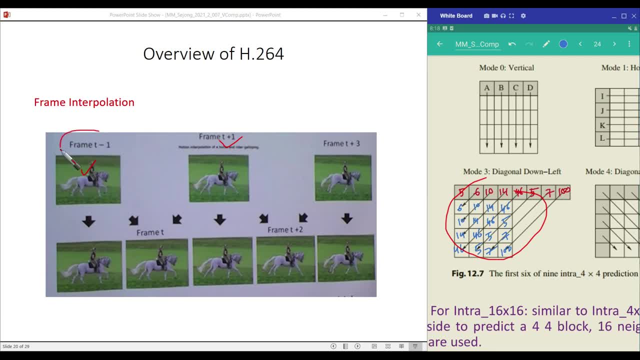 And then we perform inter-predict, inter-frame. That means you know this, using this frame and that frame, we will use this frame. So this is from when one, from one frame, we are generating another frame. 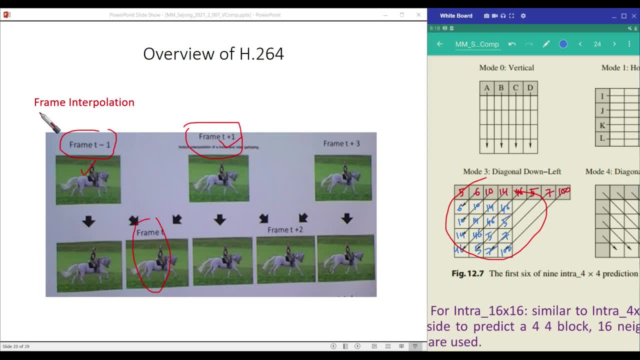 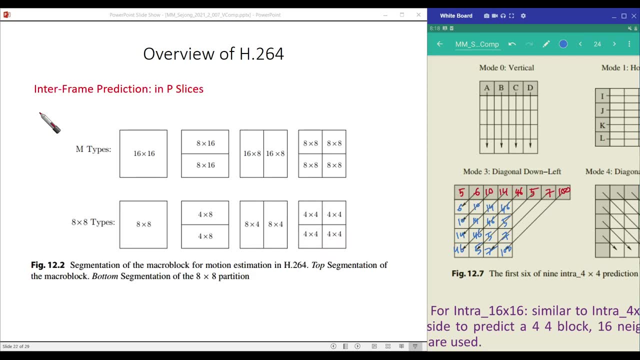 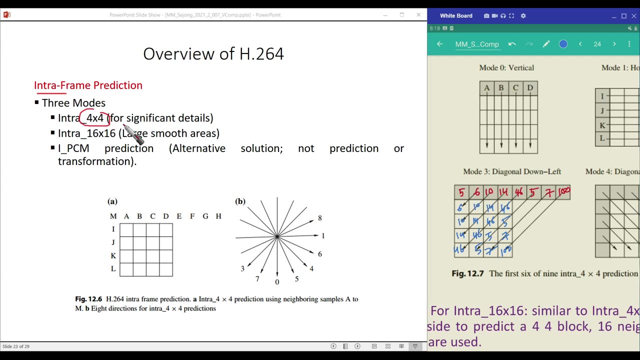 That is called, You know, frame interpolation or inter-frame interpolations, And when, within, within the frame itself, this is called intra. You know, this is called intra-frame prediction. Now we use four by four when we need, you know, significant details. 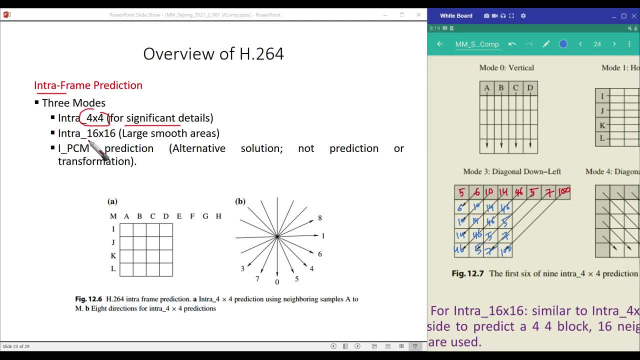 That means that you are within a small area, but we can also use you know large, a small area, Right. For example, you know not only four by four. we can basically constrict. you know 16 by 16.. 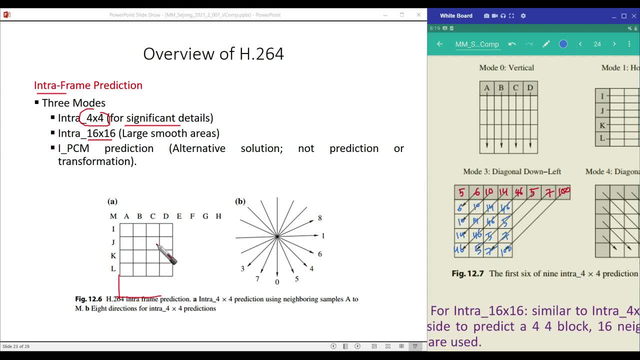 Right, 16. 16. 16. Because at that time we don't need to send, you know, lots of. for 16 by 16 pixel we don't need to send information, But definitely at that time this neighboring should also be 16 by 16.. 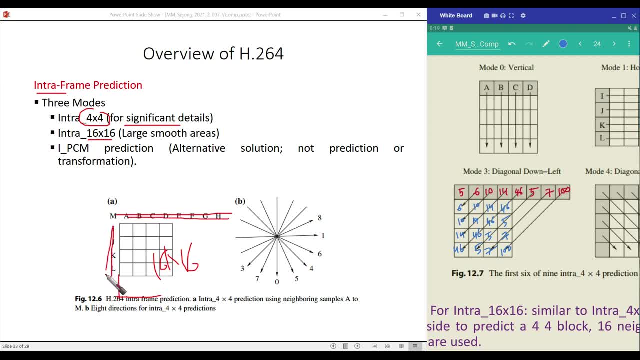 From A to up to you know 16 go, And from I to J, so you go 16 pixels. Then we can use you know this kind of you know diagrams. So this is you know one way that how this H.264 achieves better compression. 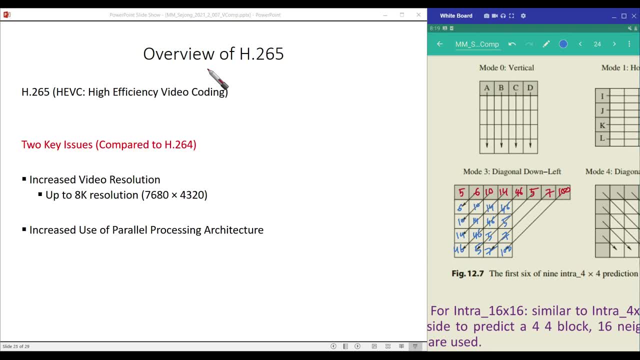 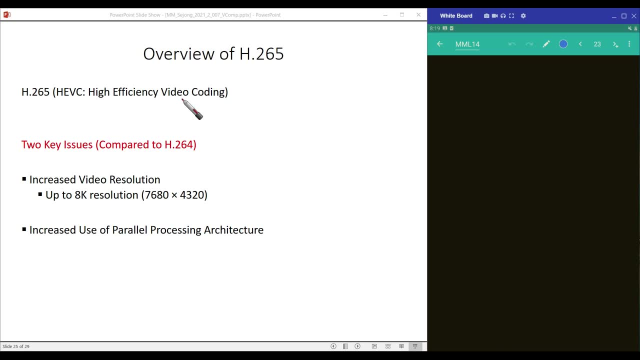 Okay, Now we'll not talk. you know more on that. Now, how about you know here H.265, this is high-efficiency video coding. You know, this is basically two key issues, the improvement compared to H.264.. 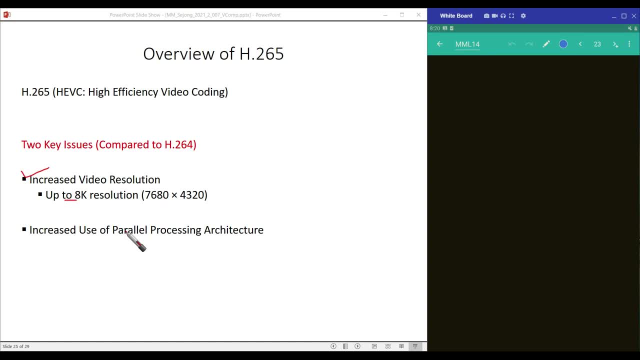 One is this: video resolution increase up to 8K And it's also introduced. you know, parallel processing architecture for high, you know for high-performance computation. So that's it. So these are some you know comparison you can read. 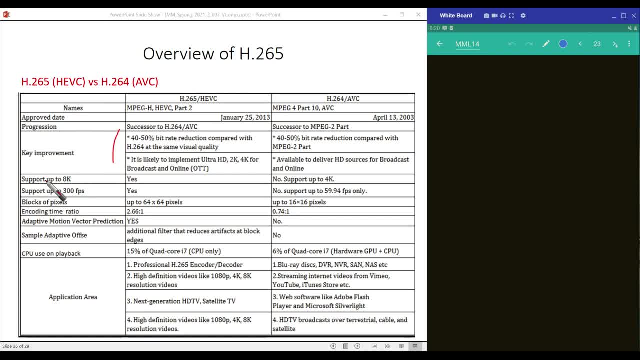 For example, this is in the key improvement. Then you have that. you know support of 8K resolution, you know bit that is frame rate, that how fast your video can be supported And how fast the encoding times can be done. 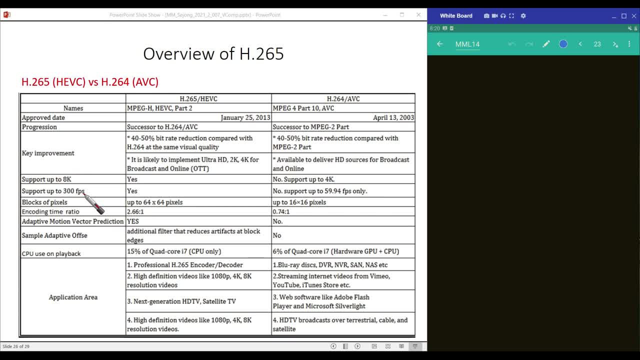 And there are various other kind of you know properties And these are the application area. So you see that H.264, that is ABC, you know. blue Blu-ray is DVR, you know, and streaming services, for example YouTube, iTunes, is still, you know, they use in this ABC. 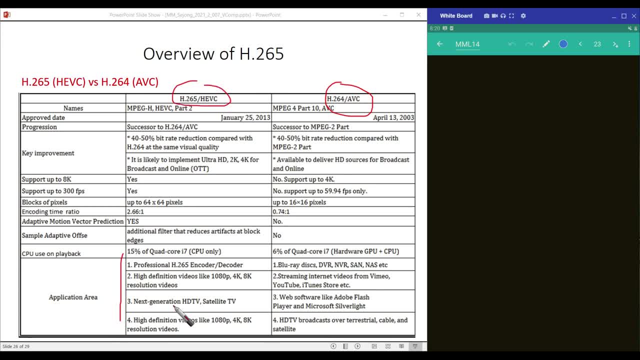 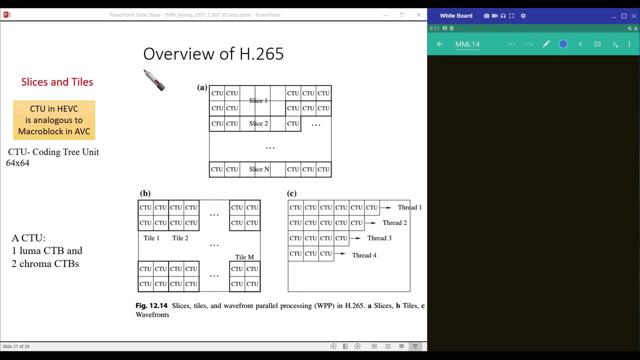 But you know H.264 is comparatively new So it's not supported, you know by, you know many recent and advanced, you know maybe the industry, But it is being adopted, definitely. So let's I talk something on that- how the parallel processing works in H.265. 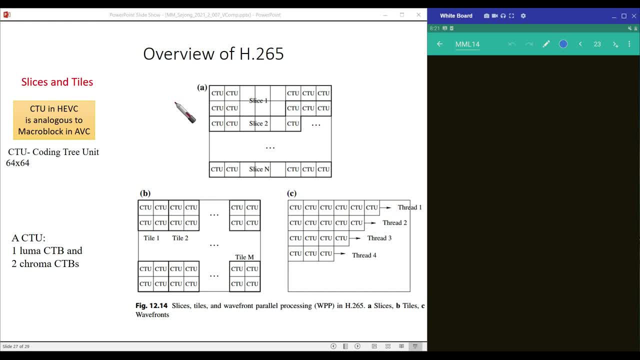 So in H.265, you know, for example, in the macro block, that is 16 by 16 macro block, 16 by 16 macro block, or let's say 8 by 8 types, you know block. 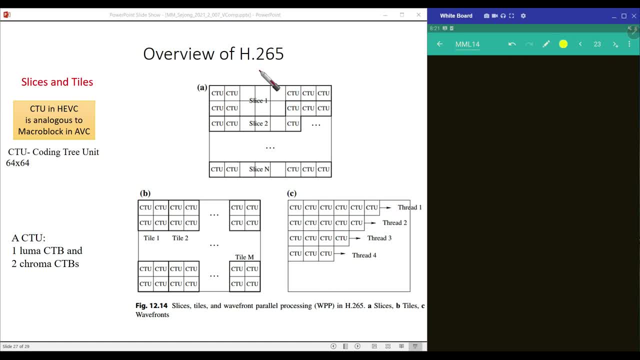 So in here, in this H.265, we use the concept called CTU. This is also, you know, kind of block. Basically this is 64 by 64, you know block, you know size okay. 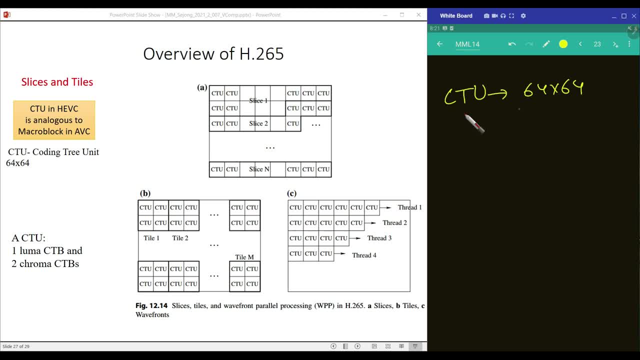 And so this is called CTU. Now, within this, you know, CTU, That is, you know coding tree unit. We say coding tree unit. okay, Now within one CTU, you know, there are definitely color information as well as brightness information, whatever. 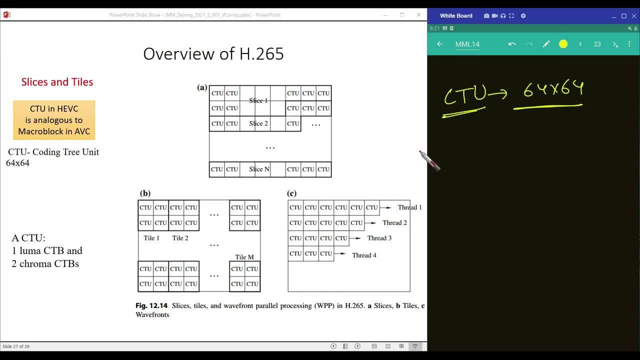 So we are not talking on that. So there are some concept. let's say, you know, parallel processing concept, One is slice concept And another is, you know, called tile concept, And we also have thread or wavefront concept. 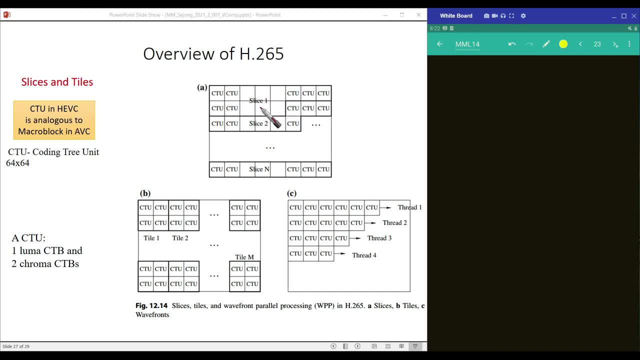 Now let's say Slice concept. Now, slice concept is, say, is that let's say this is a you know frame. Now, this single frame, we, you know, divide it into some slice. For example, this is slice 1,, this is slice 2,, this is slice N. 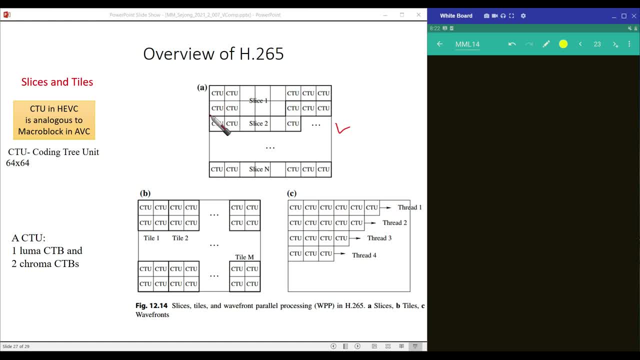 Now, when you consider the slice N, you can basically, you know, you can design the way you want. okay, So let's say, this is a slice, This is one slice, But definitely it cannot be like this. It should be like you know, some sort of you know this kind of line. 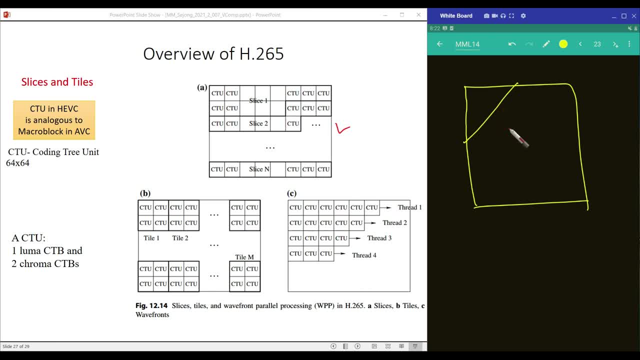 Right, Some straight line, Not, I mean, it's some how to say that You know some parallel line of this horizontal parallel line or this vertical parallel line, Because the block length is always something like you know this: either horizontal parallel or vertical parallel. 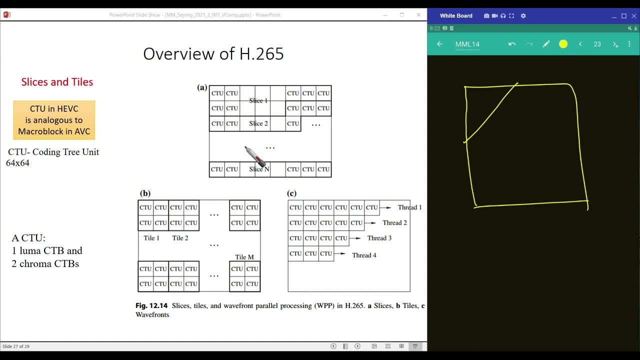 Right, Because it is square 64 by 64.. So we cannot have like this. So, rather, what we can do, let's say maybe this is one slice. Okay, Also, you may consider the slice. maybe, you know, look like that. 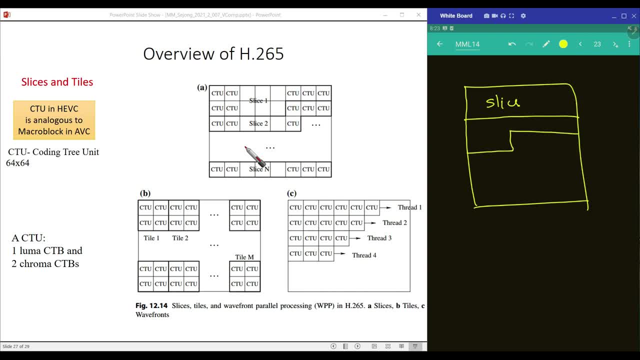 Maybe, maybe, maybe. this is, you know, Another slice Okay, So this can be a slice Okay, Or, but definitely it should be consecutive. So in this way, consecutive Or so, or in this direction, consecutive. 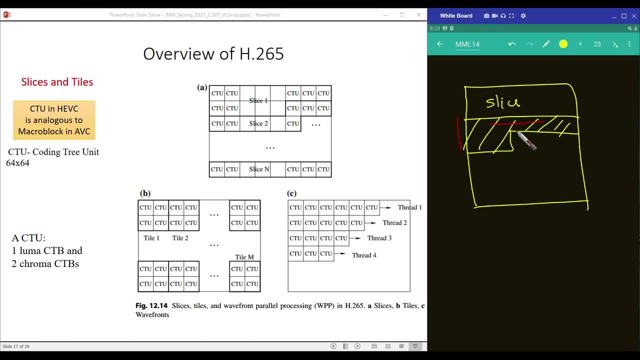 So something like that: So you cannot broke, Right, You cannot break. You know the slice should be continuous, Right? So this is what it means, So this is the slice. And then what you do. let's say, you start processing, 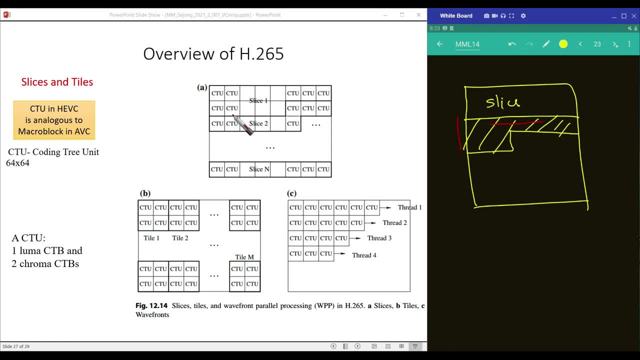 You know, for example, you do start some encoding or decoding Whatever you do, So you can. You can do some coding, you know encoding, or some operation or some processing: Image processing, So pixel processing, Video processing. 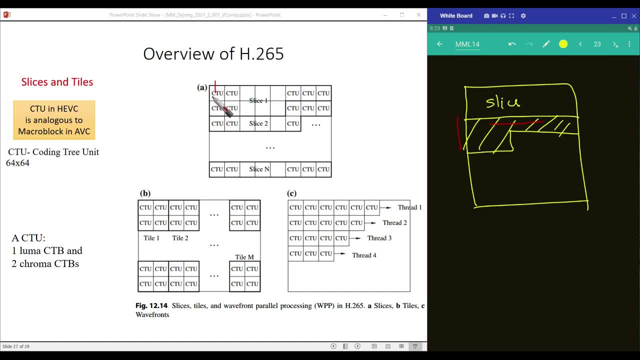 On. let's say in this unit Or so, this is block zero. Let's say CTU zero. Let's say this, very, this one, the beginning one, And then you cannot use parallel processing. 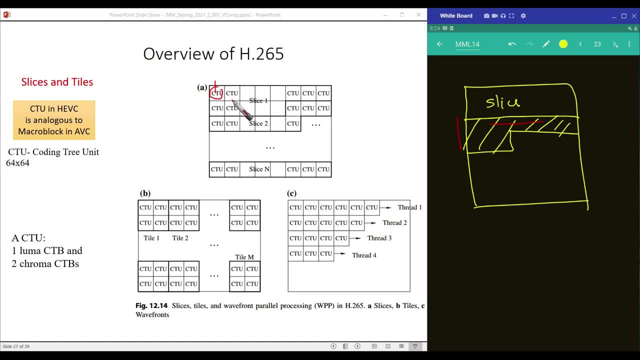 So that means the processing at the same times on another CTU in the same slice. Rather, you know, you can use maybe, you know, maybe this one And this one together, Because they this, you know CTU and this CTU coming from the different slice. 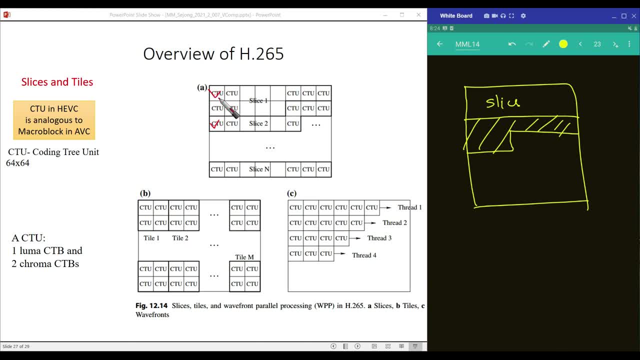 And the reason is you know, perhaps you know this CTU is somehow dependent on this neighboring CTU. This is the concept. But perhaps you know this CTU has no relation with this CTU, So we can independently process this CTU. 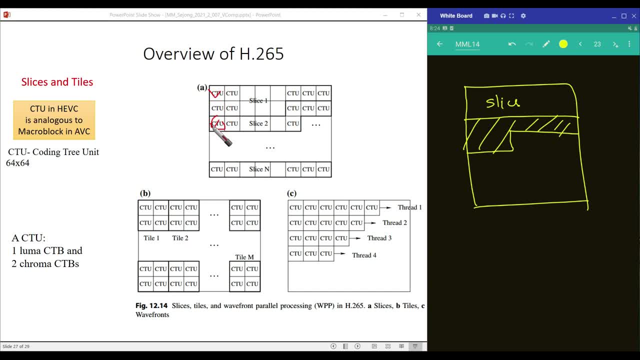 And you know the CTU is important Because you know, you know, when you have some relationship between this CPU, this CTU and this CTU, Maybe you know, maybe Because of some inter-predictions, or maybe because of some framing references. 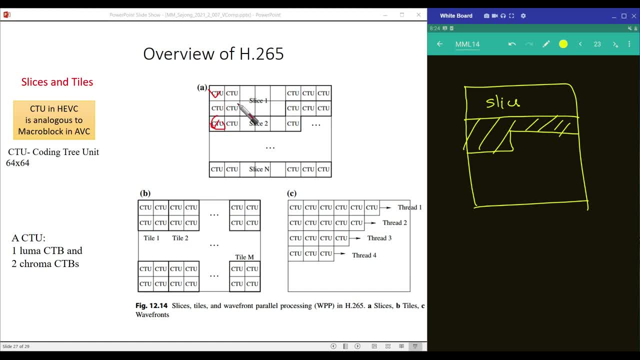 We need each other's, to generate each other's information, But perhaps you know this CTU and this CTU has no relation. So that's why we roughly say that you know we can choose any CTU from this slice. 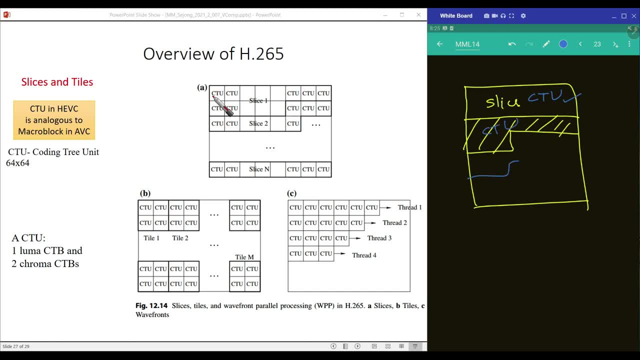 And any CTU from this slice, Or maybe this is let's say, and let's say, maybe this is you know another you know slice, So maybe then we can choose, you know. 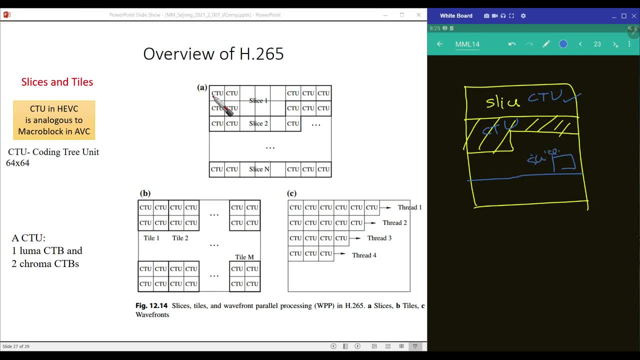 Another, you know, CTU, from this slice Right, The slice over 3.. So then we can do some parallel processing. So this is one you know idea that how parallel processing is done, And another idea is, let's say, tile concept. 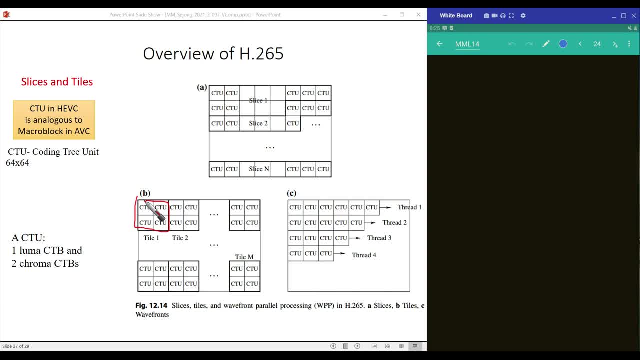 You can, rather you know, consider: look at this, This 4 CTU, you know, constitute one tile, This 4 CTU constitute one tile And this is another tile. And then what you do? you can, basically, you know, parallel process between tile 1 and tile 2, CTU. 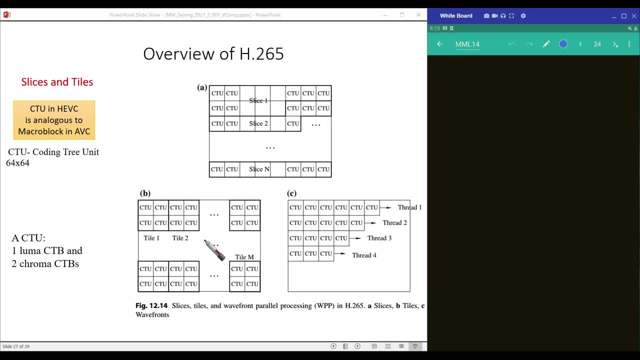 And in this way. But we can, We can't. you know, you know, do the parallel processing between this CTU and this CTU, Because they are coming from the same tile. Then you also have the concepts of you know, thread concept. 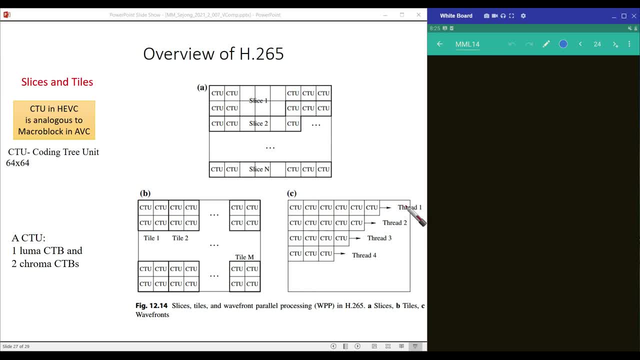 This is like CPU concept, Right, That, for example, that let's say this: CTU, you know this. in this line, they consider thread 1.. This is thread 2.. This is thread 3.. This is thread 4.. 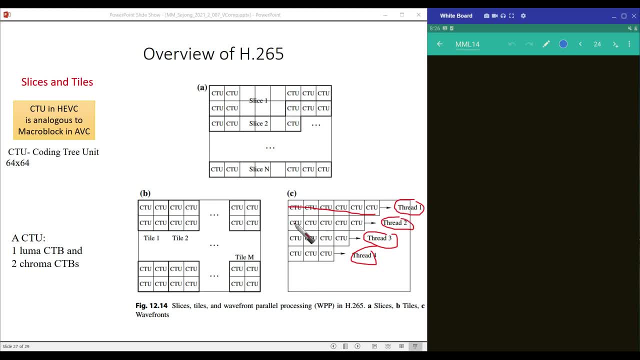 What we can do. basically, we can take CTU from thread 1. And at the same time we can take, you know, another CTU from thread 2. And we can do some parallel processing. So these are you know different kinds of, you know concepts of parallel processing that you know are used here. 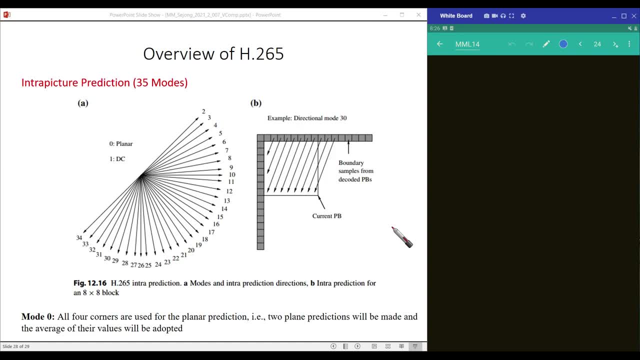 Okay, Now this is called from computational perspectives And from compression perspectives. you know, H.265 use 35 different modes of for intra-frame predictions, That is, within the same frame, you know it- as if different kinds of direction. 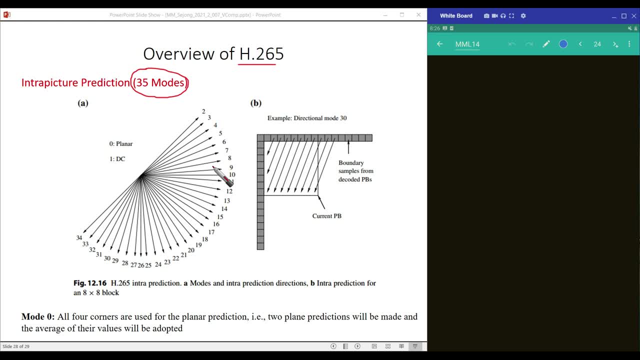 That means every possible. you know redundancy, You know we exploit here, And this is from mode 0 to mode 34.. Okay, So mode 1 is simple DC. So that means you just do average, for example here: 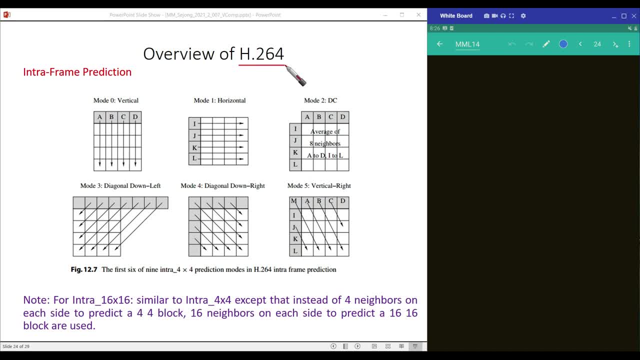 If you go- this is more, for example in H.264, if you use mode 2, that is DC. So that means, in this mode you basically, you know, take values A, B, C, D, I, J, K, L. 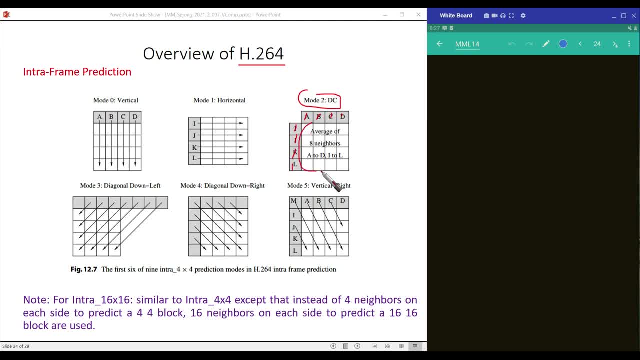 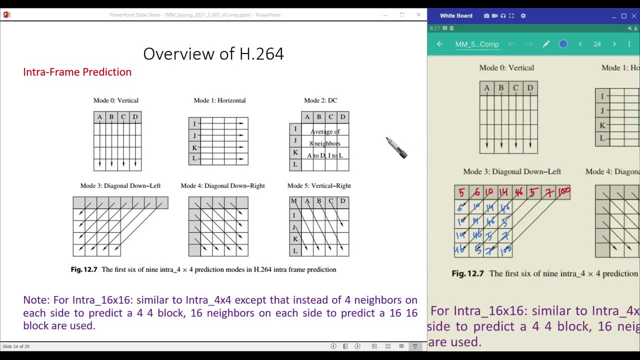 And then you make average of all of these And you use the same values here, Right? So this is called DC operation. You are just taking average, If I just go back, for example, here, So you can imagine that what we mean by this. you know DC1.. 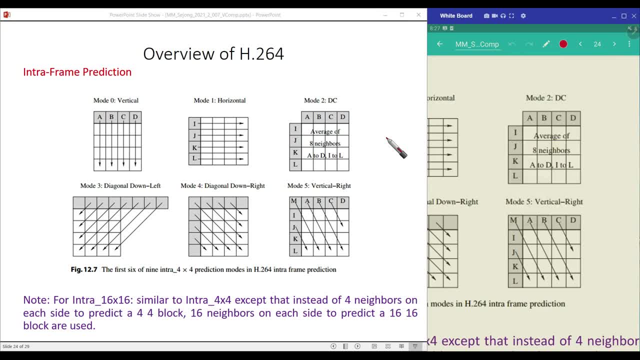 You can easily understand. For example, if we have, you know these values, let's say 4. These values, let's say 3. These values, 5. This is 6. Let's say this is 7.. 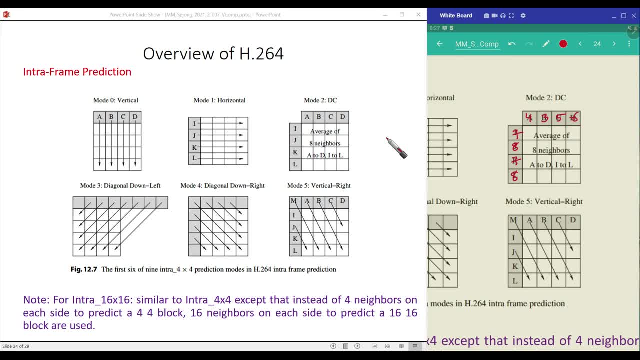 This is 8.. This is 7.. Maybe this is 8. So then, what So? the total? you know, 4 plus 3 is 7. Plus 5 is 12. 18. 25.. 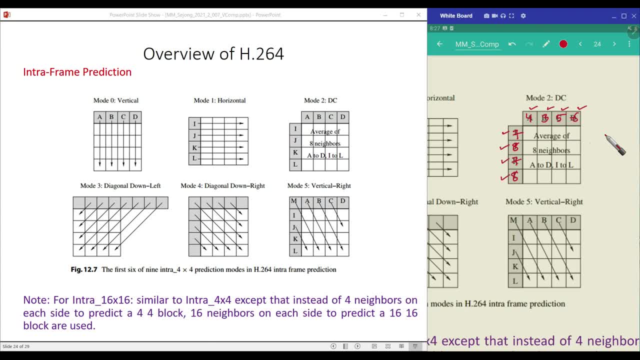 And then 43., 50., 58., Right? So then you just take the 58. Divide it by 8.. So maybe you know 7 point something, Right? So then this 7 point something basically uses 7 point something. 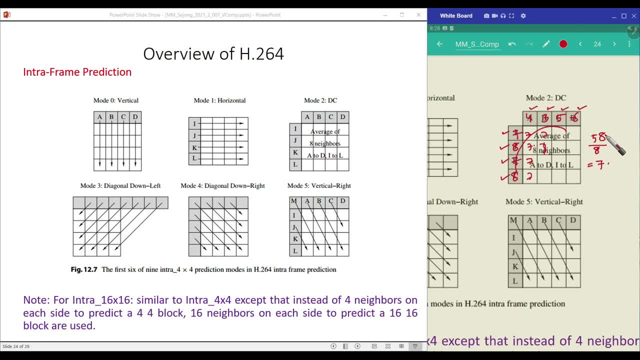 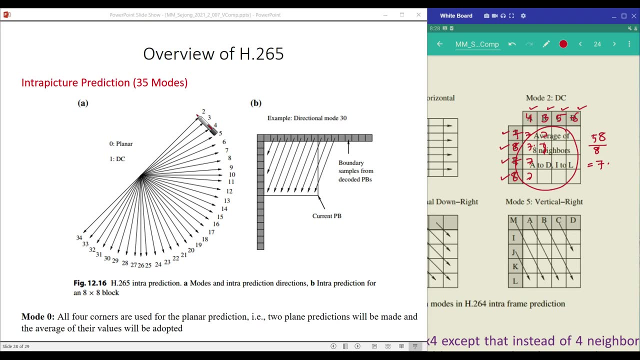